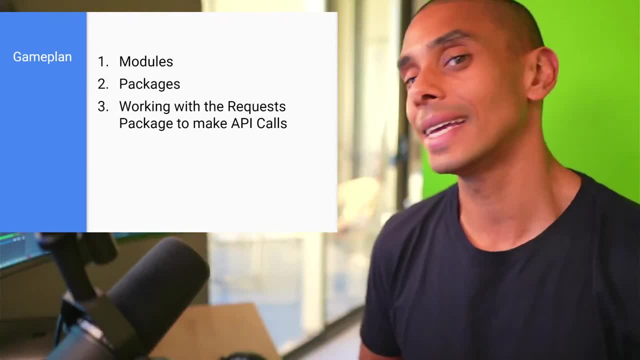 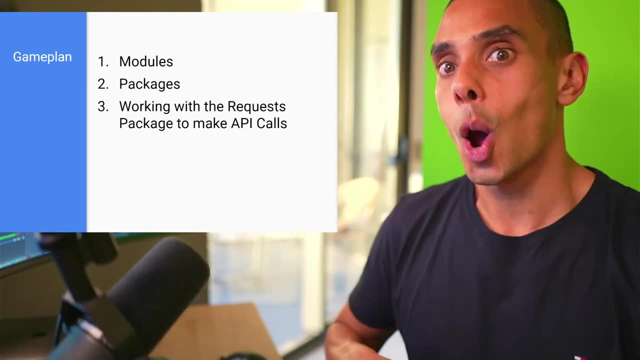 your code and store it inside of a separate file and bring it into your Jupyter Notebook. So we'll take a look at how to do that. today We will also be touching on packages. So packages open up a whole wide world of opportunity when it comes to doing data science with Python. And then what? 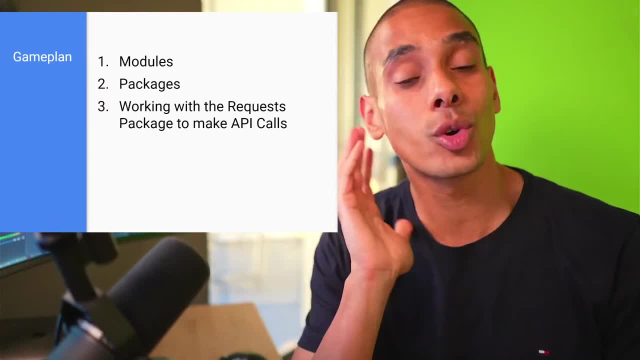 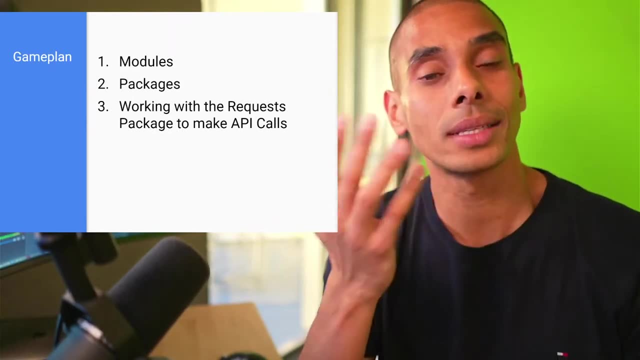 we're also going to be doing is we're actually going to be using a specific package called the request package. So the request package actually allows you to make API calls to just about anything around the web. So we'll actually test this out on a couple of my favorite APIs that we 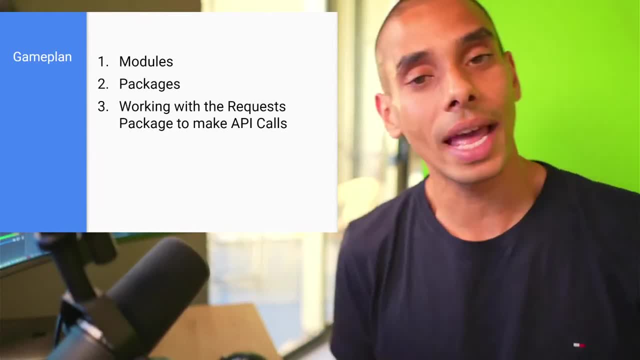 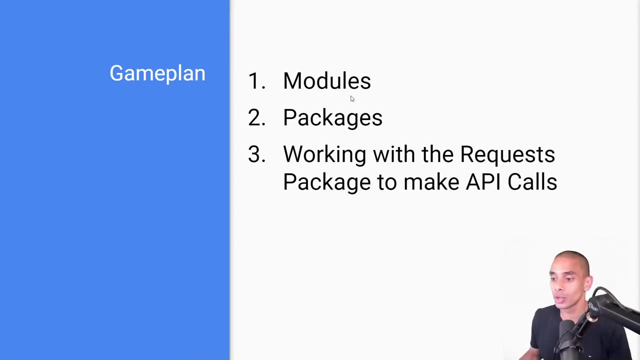 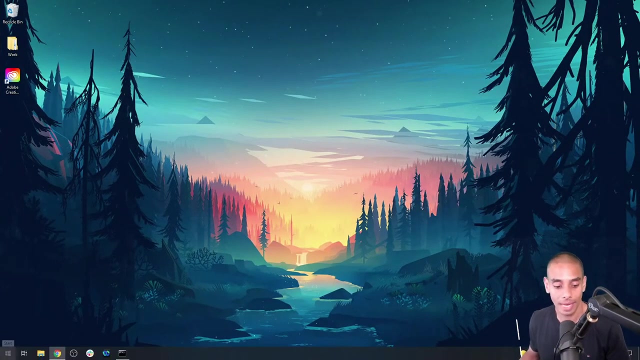 can actually access relatively easily. So, on that note, let's actually kick this thing off. So the first thing that we're going to do is we're going to start out as per usual. We're going to go on ahead and open up our Jupyter Notebook, And so I'm going to navigate to where my Jupyter Notebook 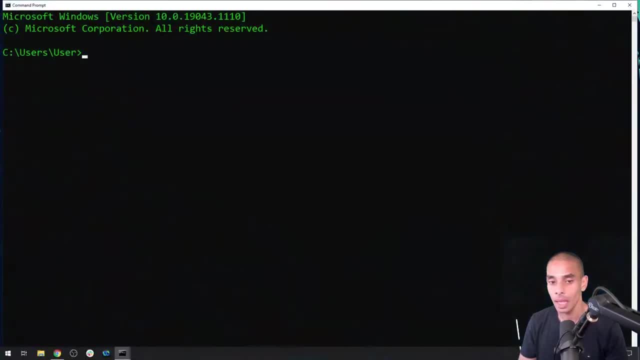 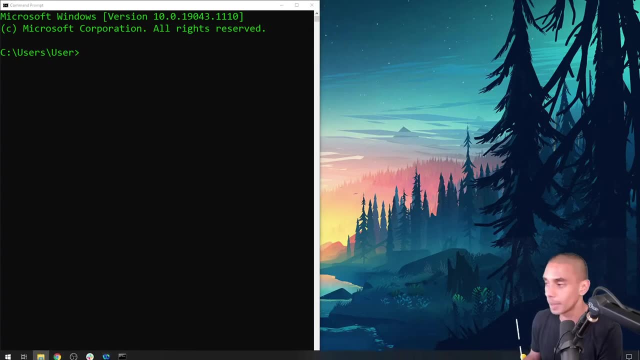 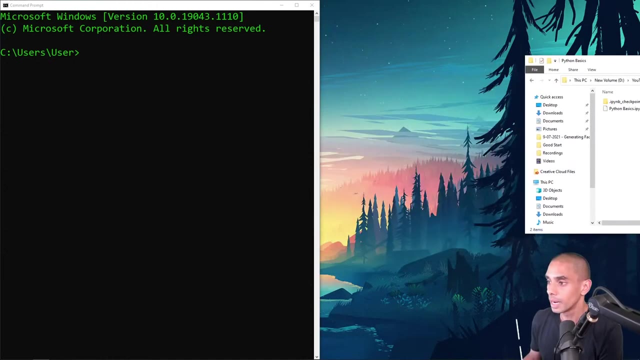 currently is, So we can just type in cmd And remember: our Jupyter Notebook that we've been working with so far is inside of a folder called- I believe it was- Python basic. So let me open this up And let's just show you where it is Right here. There it is. Let's bring that over there, Cool. 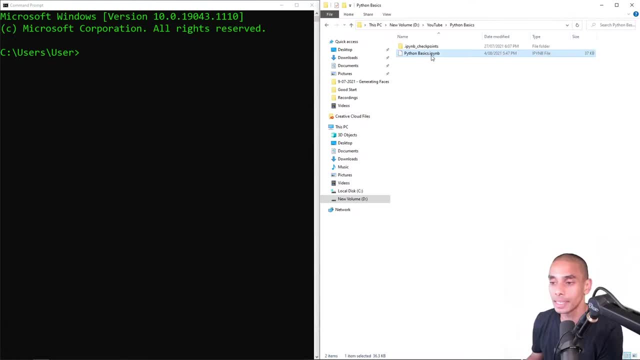 Alright, so you can see that inside of our folder we've got a Jupyter Notebook called pythonbasicsipynb. So what we can do is we can go into that and open it up, as per usual. So we're going to cd into there. 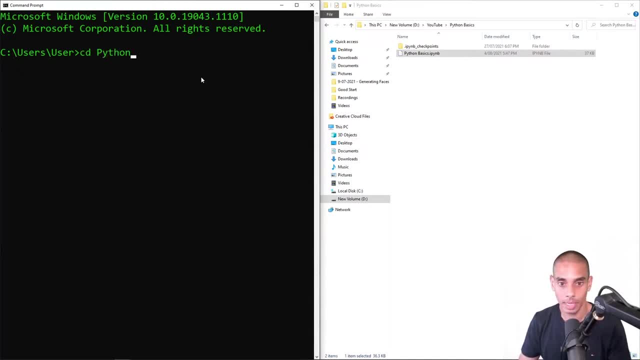 cd python basics. We need to go into our D drive first, a D drive, CD YouTube, CD PythonBasics. And what we're going to do is we're going to go into that and open it up, as per usual. So we're going to cd into there- CD PythonBasics. 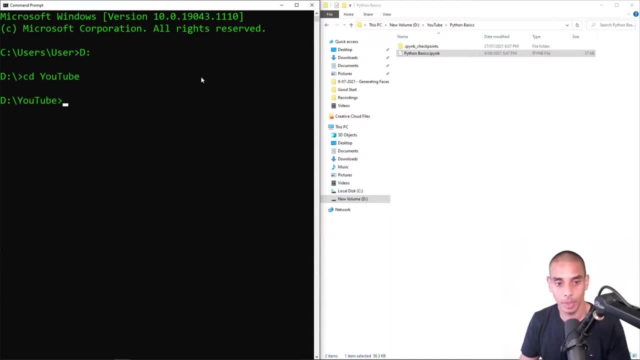 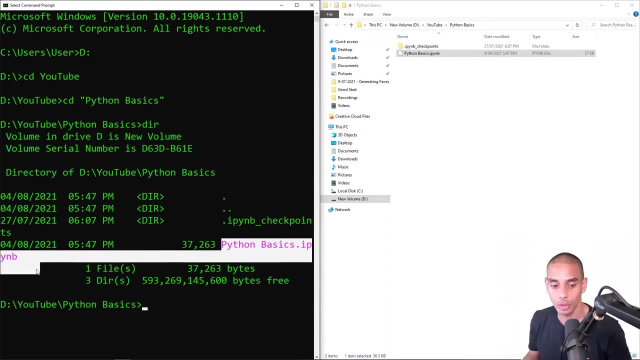 We need to go into our D drive first. So D drive, cd, YouTube, CD, PythonBasics, python basics. and if we take a look inside that folder, we can see that we do in fact have our jupyter notebook there. so python basics, dot, ipy, nb. so what we're going to do is we're going to 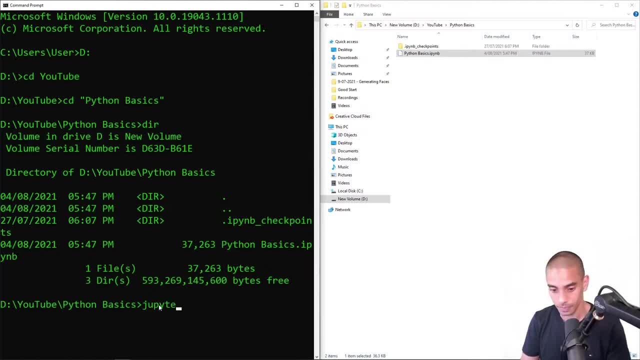 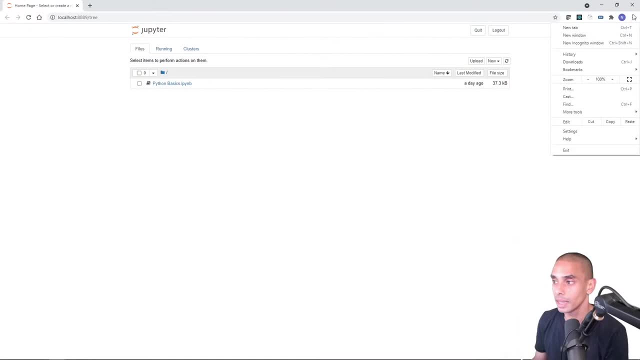 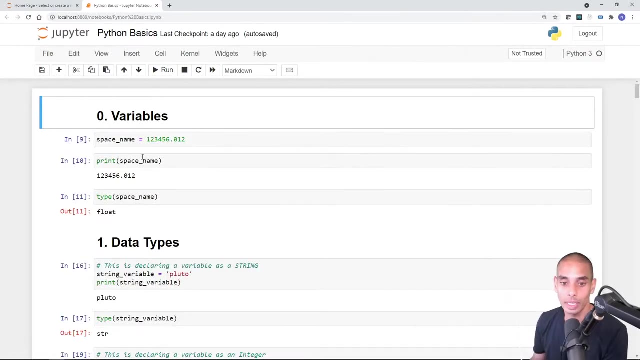 start up jupyter. so we can do that by typing in jupyter notebook and this will open up jupyter notebook and you can see we've got that there. let's zoom in to make it a little bit easier to see. and if we open up our jupyter notebook we're going to have a bunch of stuff available inside. 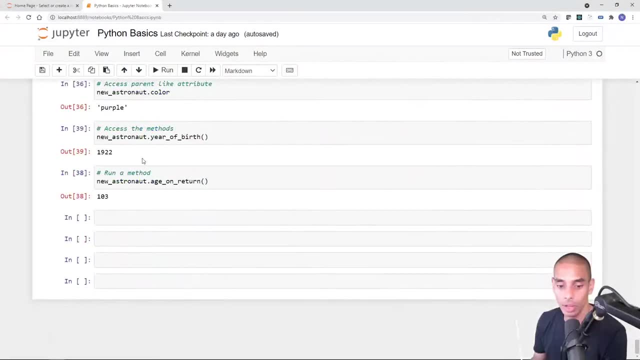 of this. so we are now up to our next section. so we're going to scroll on down and again, all of this code is going to be available once i finally get it together, so you'll actually be able to pick this up and use it all yourself. so what are we going to do? we're going to add a couple of extra. 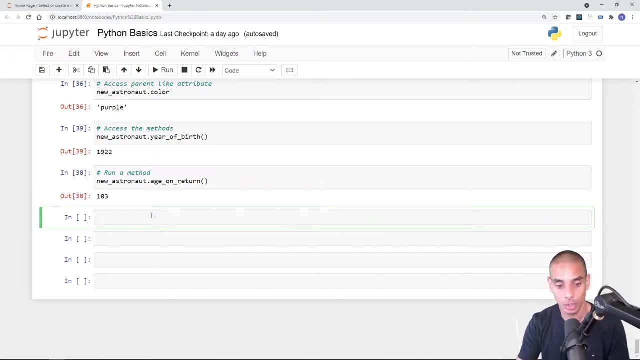 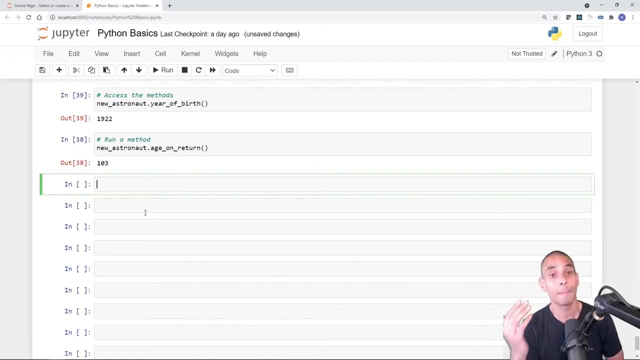 cells. now remember to get outside of a cell, inside of jupyter. we just hit escape to convert it from green to blue. add in a bunch of additional cells by hitting b on our keyboard. remember b adds cells below our current cell. so if we wanted to add cells above, we can select a different cell and 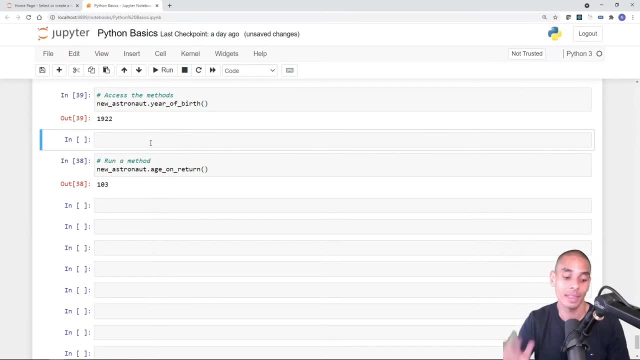 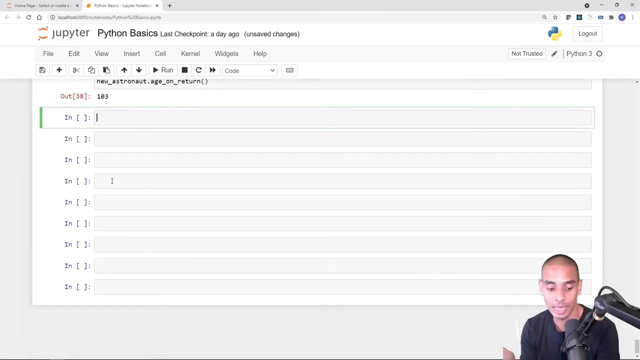 hit a and that will add a cell into or above the current active cell to delete that cell. we can hit dd to delete that. now, as per usual, what? what we've been doing in this series is we've been starting out each section with a separate markdown cell. so to do that again, we're going to hit escape on our 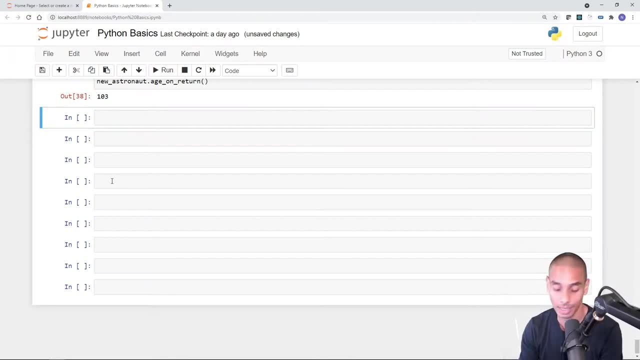 keyboard and convert this cell here to m or markdown. so i'm going to hit m on my keyboard and you can see it's converted it to markdown over there. now we are going to name this section. what are we naming this? we are going to call it modules. what are we currently up to? we're up to 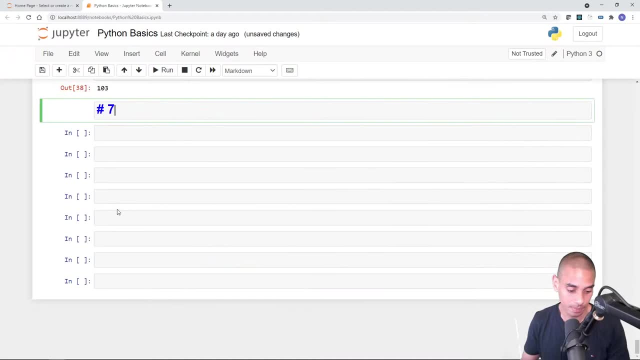 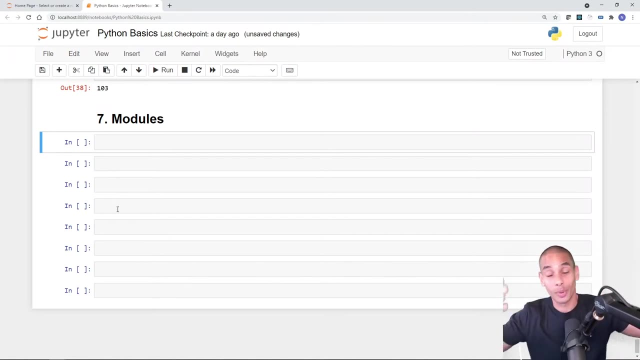 set six, so we're going to call this section seven modules. all right, now i want to put you, i want you to put yourself in the hot seat as a data scientist. so say, you've written a bunch of code, you're using it often, or you're using that exact same code often and often, and you don't want to have to. 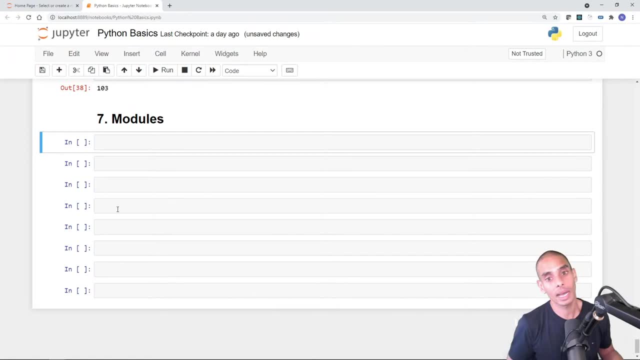 go and write it again inside of your jupyter notebook. it'd be so much easier if you could just import this or inside from another file so that you can use it just about anywhere. well, this is where modules come in handy, right? we can actually import code that we have inside of another file. 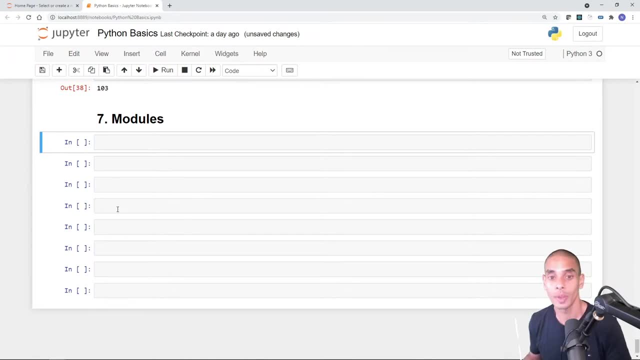 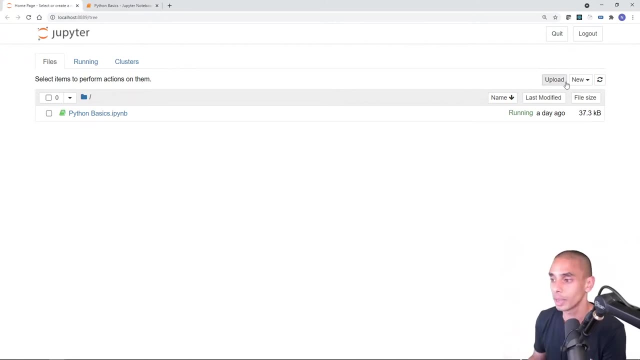 into our existing python script or into our jupyter notebook. so the first thing that we want to go on ahead and do is actually create a separate python script. so let's go ahead and do this. i'm going to create a new text file. can we save this? we can't say this is jupyter. let's. 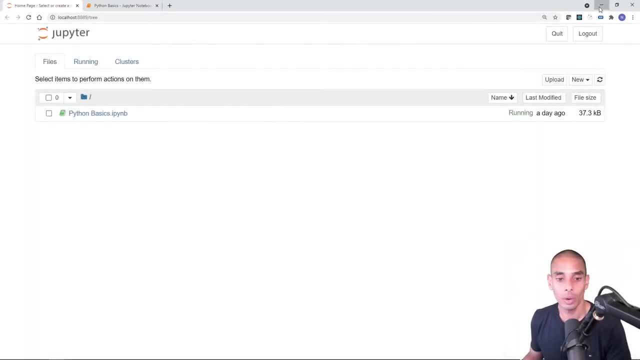 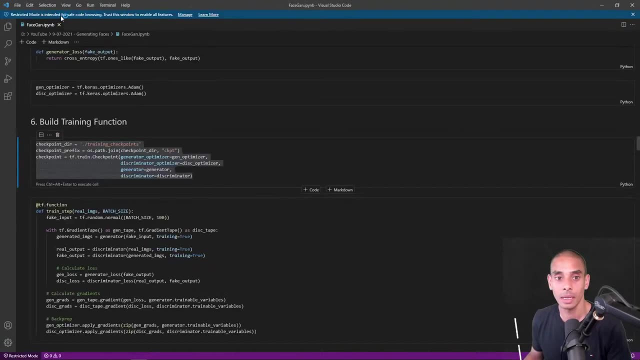 go ahead and create a new python script, so let's delete this. let's go and open up vs code or your favorite code editor. so i'm going to open up vs code in this particular case, and what i'm going to do is i'm going to create a new python script, so we're going to hit. 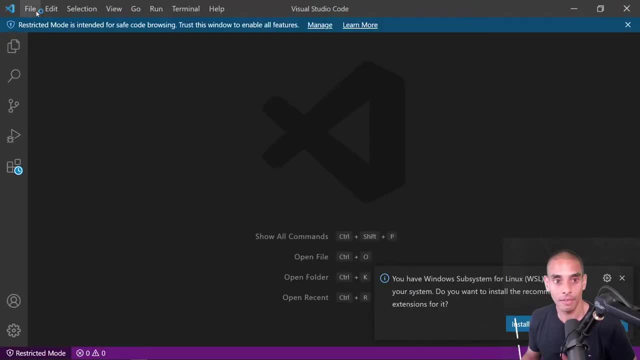 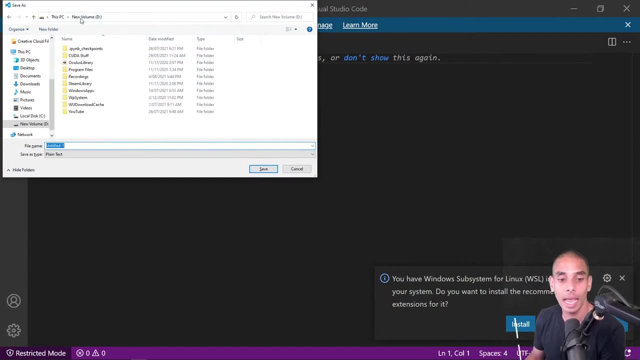 let's make this a bit bigger. so i'm going to hit file, new file and we are going to call this. so let's actually save it now. we're going to save it in the same folder that we're currently working in and i'm going to call this: uh, helpers. all right, so we're going to call our file helpers, dot pi. 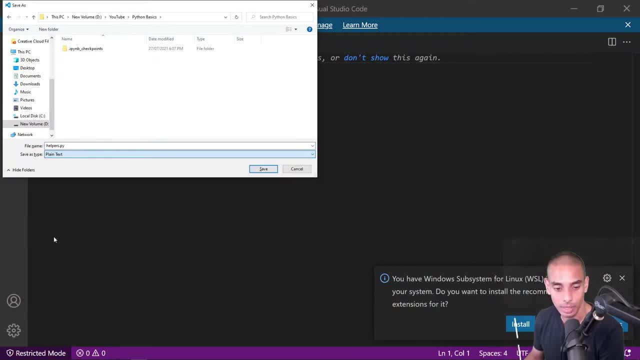 and we are going to save it as a python script. so down here, right. so what we're doing is we're creating an empty python script and we're calling it helpers and we're saving it as a python script. so if i hit save now, you can see that we've got this little python symbol up here and it's called. 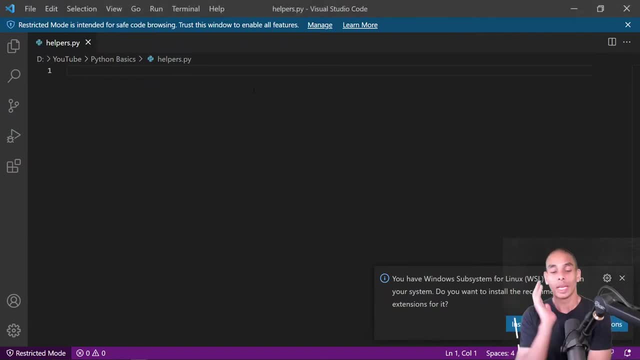 helpers dot pi. now what we're going to do is we're going to create a function in here. so say, for you write a bunch of code. this is code that you use often and often and often again and you want to be able to bring this inside of your jupyter notebook. so we're going to store some helpers now. 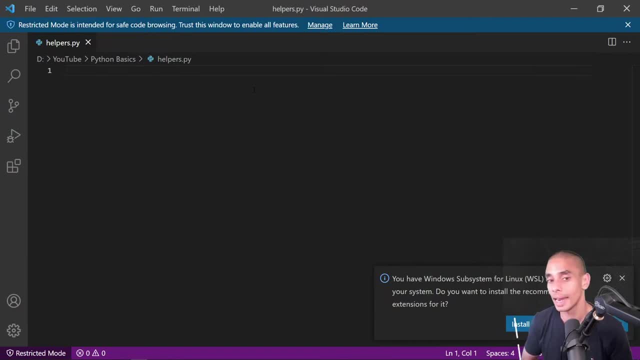 let's just say that we had like a unique number that we wanted to set as our random number inside of our python or jupyter script. what we could do is we could create a function again. we create a function by typing d, e, f, and then we can name it anything. so this function is: 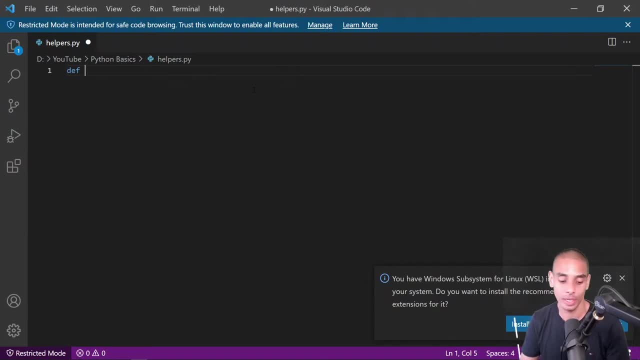 going to store our unique launch codes for our space shuttle again, so we're going to call it launch codes and then this particular function is just going to return a number, so we're going to return one, two, three, four, five, six, seven, eight, nine, super secure right. and we're going to comment this. 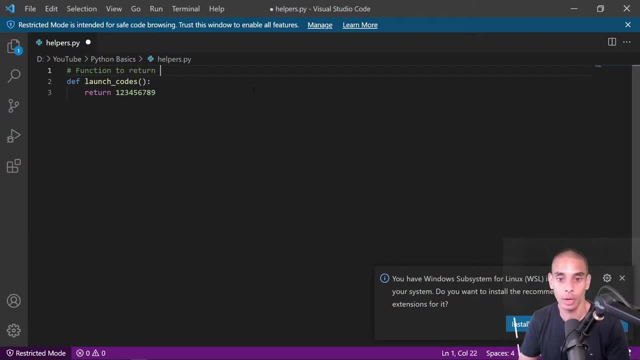 return function to return launch codes. right, so what we've gone and written there is inside of our helpers dot pi file. we've written d, e, f to define a new function. we've then called that function: launch underscore codes. and then we're going to call that function launch underscore codes. 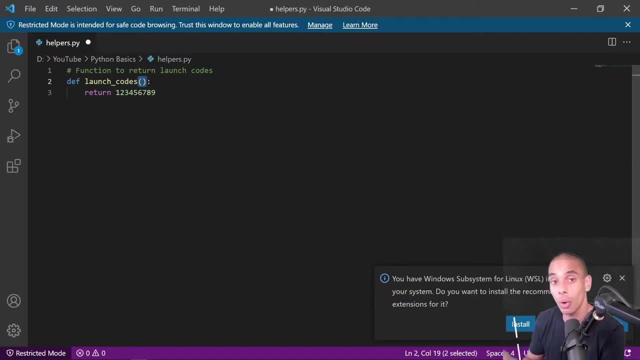 and then we've set a set of parentheses so we're not passing any positional or keyword arguments. we've then passed through a colon and this function is going to return the number one, two, three, four, five, six, seven, eight, nine. so this is an integer in this particular case. 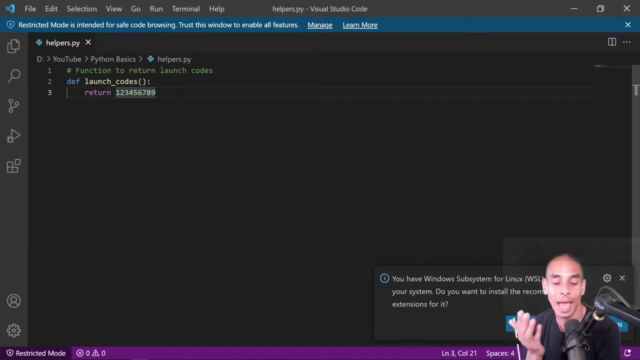 we can then save this. so right now, we haven't actually done anything with this helper code, right? so we've just got this blank, uh piece of code, but we can't actually do anything with it. but what we can actually do is we can actually bring this into our jupyter notebook. so how am i? 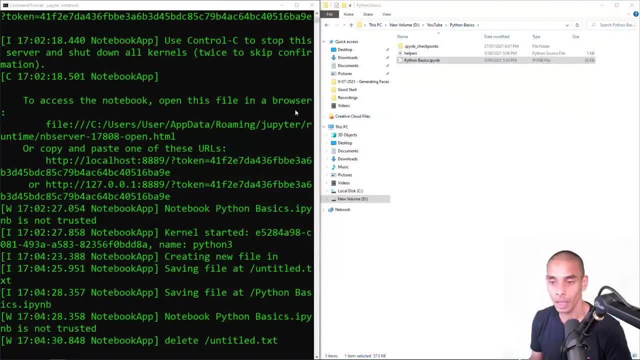 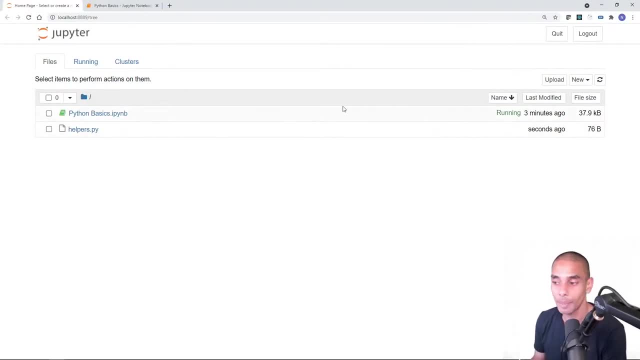 we go about doing this. i'm going to close this for now and we're going to open up our jupyter notebook again and you can see that helperspy is now showing up in our same folder structure inside of jupyter. so i'm going to step back into our jupyter notebook and then what we 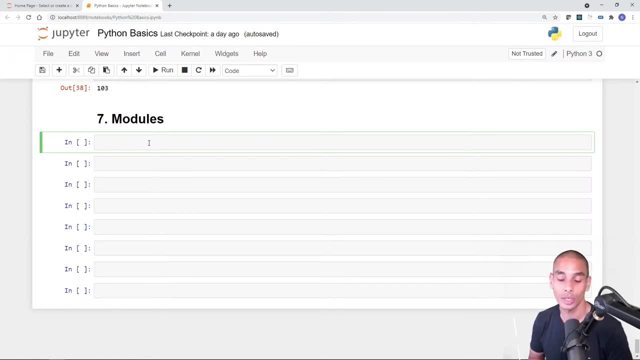 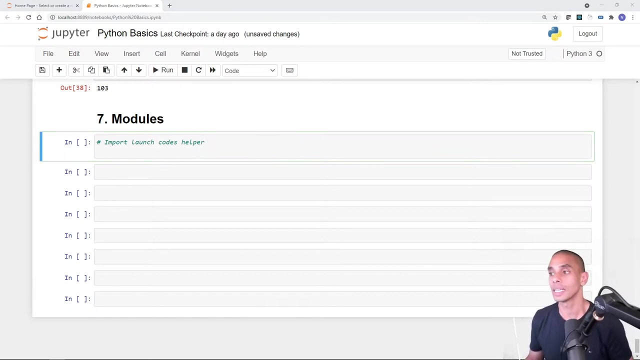 can actually do is we can actually import that launch codes function into our jupyter notebook. so let's go ahead and do this. so i'm going to create a new comment. so import launch codes helper or launch codes helper- yeah, that sounds about right, and then we can actually import this into. 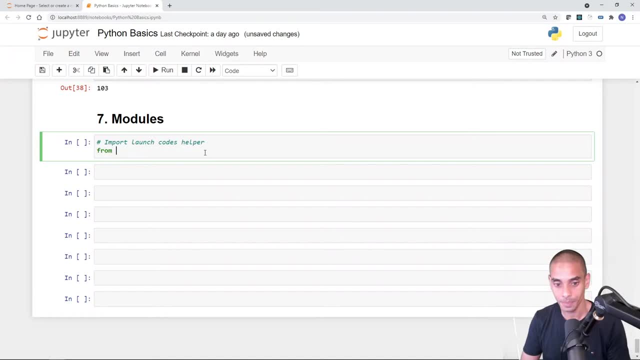 our jupyter notebook. so let's go ahead and do that so i can write from helpers, because that's the name of our file import, and then if i hit tab it's going to show what available functions i've got to import into my jupyter notebook. so this will show functions, classes, whatever you've got inside of. 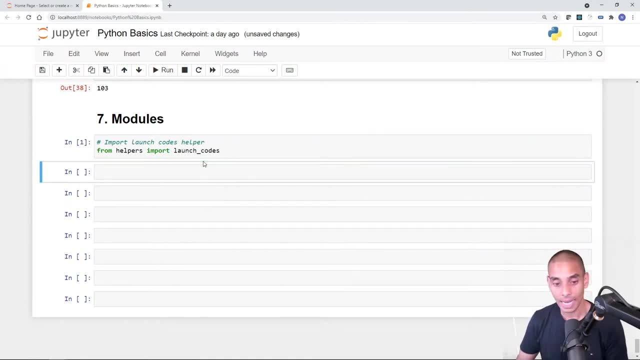 that file. so in this case i can hit launch codes, and this has actually allowed us to import our helper module, and specifically one function from our helper module, into our jupyter notebook. what we can then do is run the launch codes method, so launch underscore codes. launch codes function actually, and you can see that we are now returning our unique launch code. 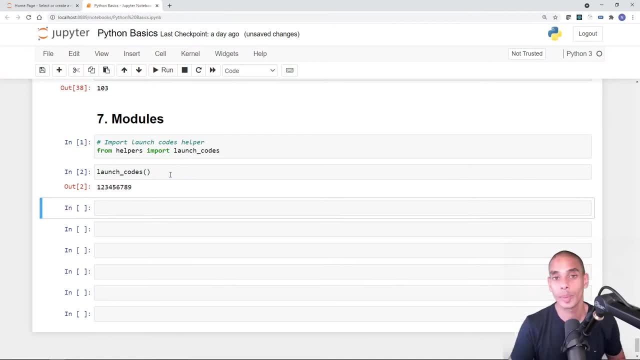 number. so, again, this just makes it really really useful, particularly when you're building up huge data science workloads. having specific modules or helpers stored inside of separate files makes your life a ton easier, rather than doing everything inside of one massive notebook. and again, notebooks are really flexible, so you could definitely do it in a single notebook. 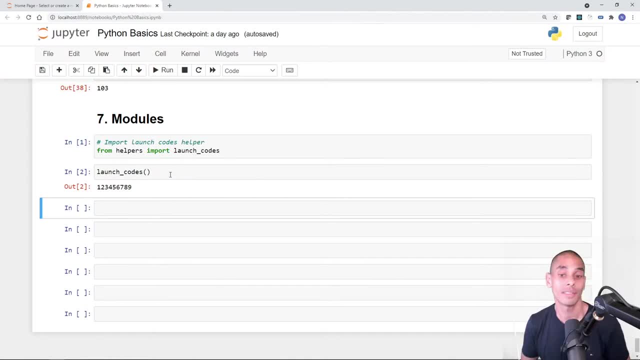 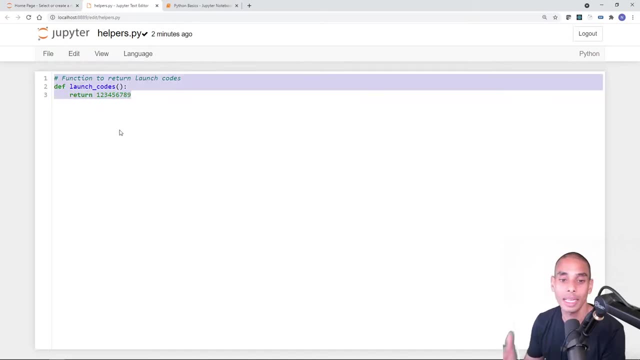 but having some of your helpers outside in modules definitely helps. so let's quickly recap on what we did there. so we went and authored our helperspy file inside of vs code and we created a function called launch underscore codes which returns the value one, two, three, four, five, six, seven, eight, nine. 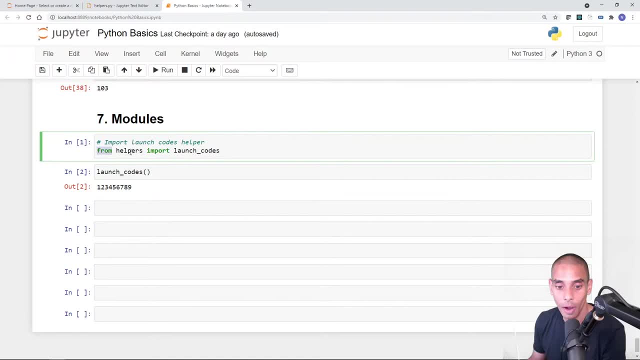 and then, in order to import that into our jupyter notebook, we can just write from helpers, because that's the name of our file, import launch codes, because that's the name of our function, and then we can just go and run that function as per usual. so that, in a nutshell, is modules now done. now you 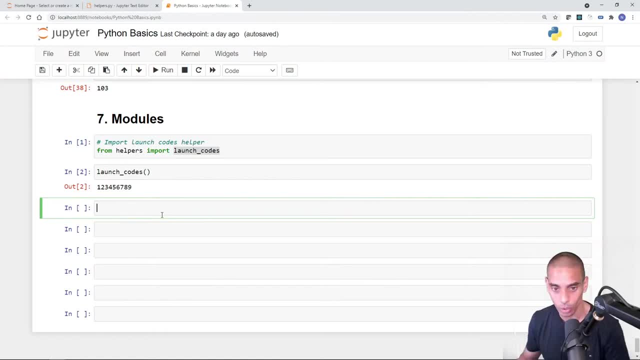 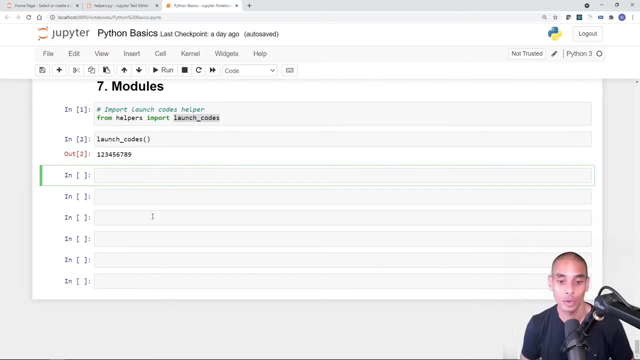 probably think you, nick, that's great, but what i'm not? i don't want to have to go and write every single module or every single function that i want to go and use. there's just way too many. well, this is where the python package repository comes in handy. so if you actually go to pypi, 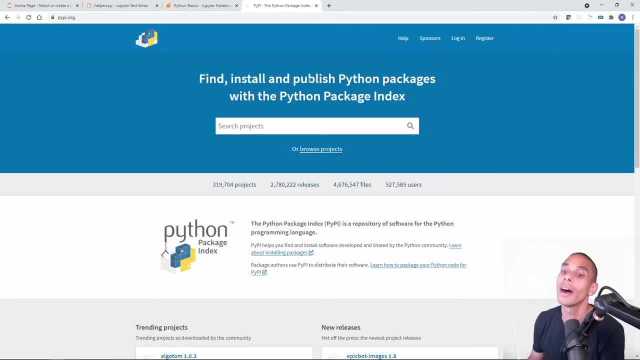 org, you will find that there are a ton of python packages that are available for you to pick up, that you can actually access from the global repository. so this is the collective knowledge of all the amazing python developers out there that you can tap into and get started using. 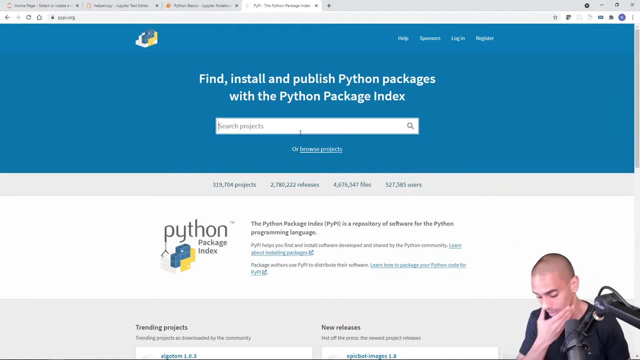 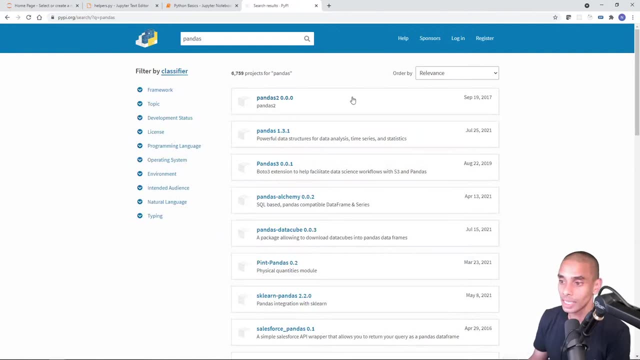 so in this particular case, or wallet, let's actually take a look at a couple. so some of the most popular ones when it comes to data science are pandas. so if you type in pandas, you can see that we've got pandas from here. another one that's really, really popular is 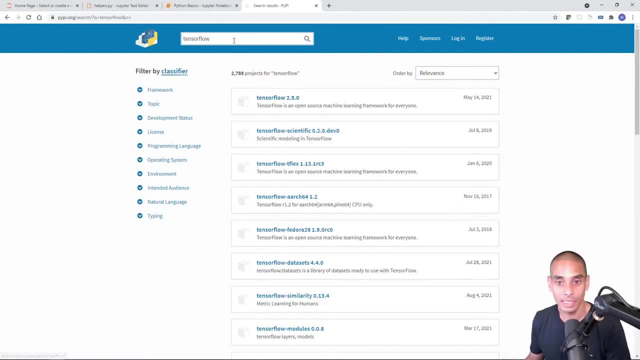 tensorflow so you can see, we can download tensorflow from here. uh, what else is there? so there's numpy. so numpy allows you. so pandas, let's actually take a step back. so pandas allows you to work with tabular data really, really easily. tensorflow allows you to build deep learning models. 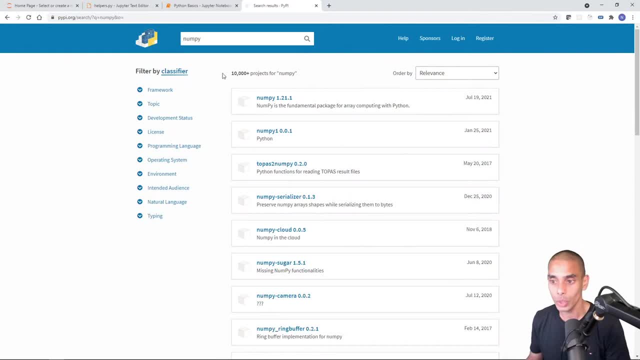 another super popular one is numpy, which allows you to work with array functions or work with some other libraries. um, so we've talked about lists quite a fair bit, so numpy allows you to work with specific numpy arrays. they're sort of like lists but they're wrapped up inside of. 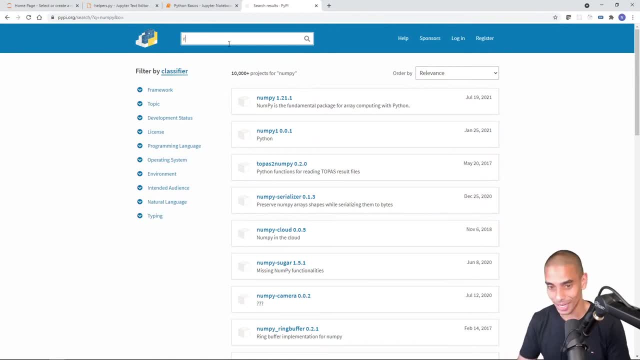 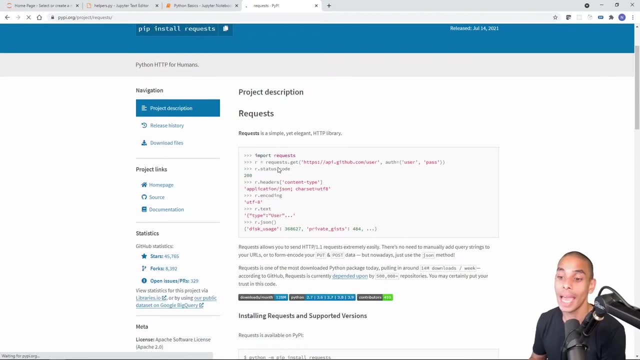 our numpy classes. another super popular one which we're actually going to use is called requests, and requests actually allows you to make api calls. so when you think about using api calls out in the wild- so sometimes when you're a data scientist or when you're working in- 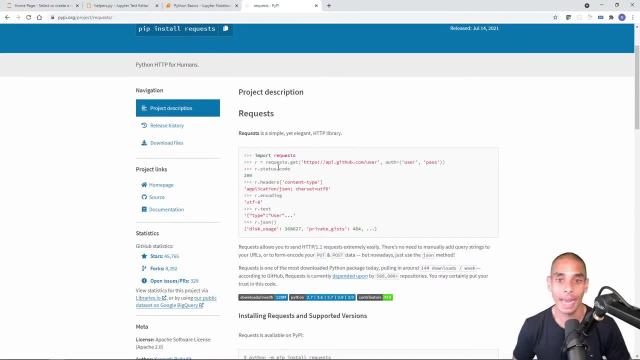 data analysis type projects, you might need to grab some data data via an api. well, the request library is going to make your life a ton easier, and it's actually reasonably straightforward to be able to use an a or call an api via request. now, if you haven't. 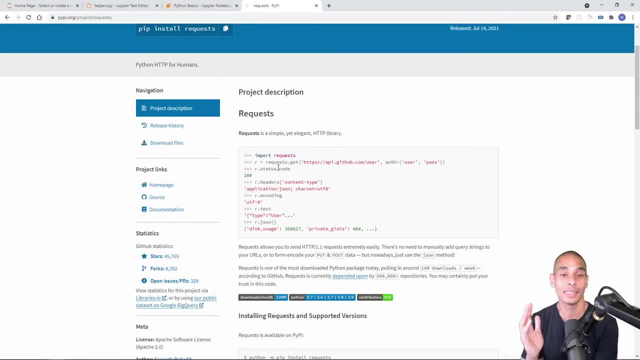 encountered apis before. if you don't know what an api is, it stands for application programming interface. now, the best way to explain what this is is that it's a remote url, so sort of like httpgooglecom. it's a remote url that allows you to call it and return a specific value. so one of, or a couple of, 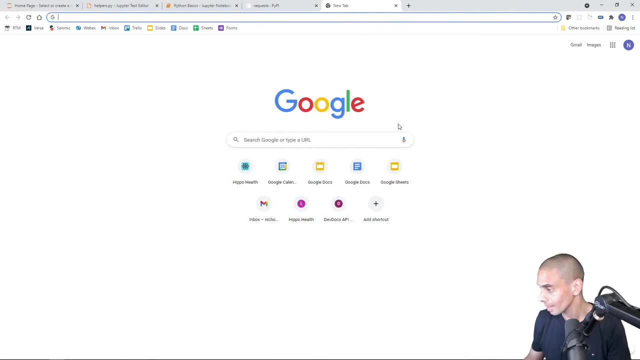 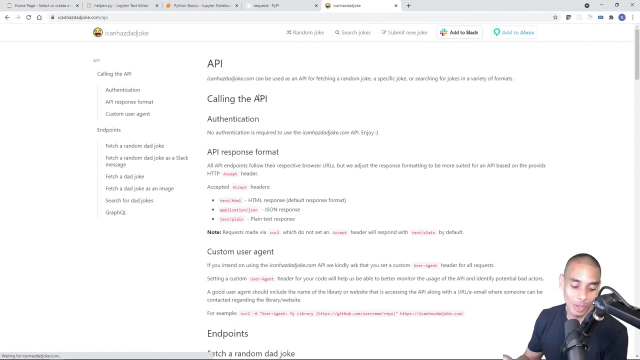 my favorite urls are: what were they? again, i had them written here so i can has a dad joke, i can has visit dad joke. so this is an api. again, it's not super data science specific, but i sort of wanted to make this a little bit fun. so this actually is an api that allows you to call it and return a specific. 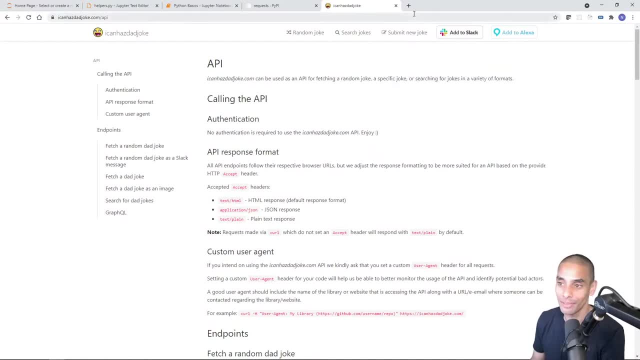 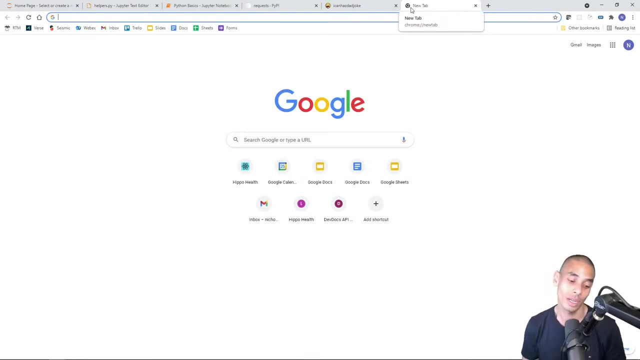 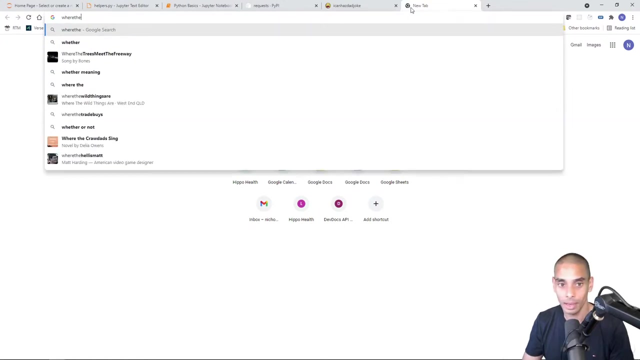 value that allows you to return or fetches a random joke from a variety of formats. another one, which is a little bit more data centric, is an api that actually allows you to get the location of the international space station at any point in time. so the api for that is where the iss. 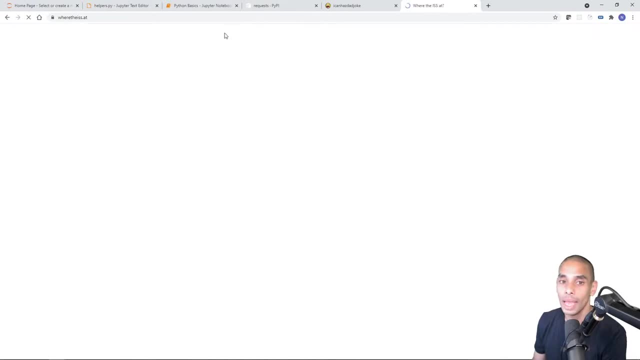 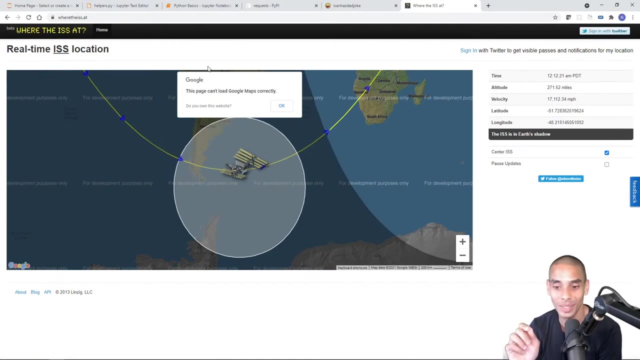 got at, and so there's actually a huge api that sits behind this that allows you to track where the iss is at a given point in time, which is pretty, pretty cool. so this is a huge api that allows you to track where the iss is at a given point in time, which is 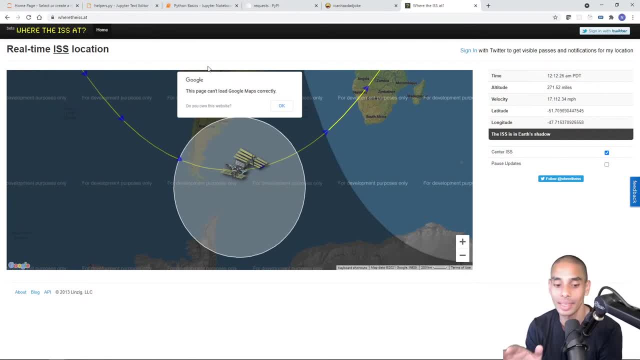 this is the main page, but there's actually a whole api that sits behind this that we can actually go and hit to be able to bring into our jupyter notebook and work with it. now these are just two examples that i like taking a look at, but there's a whole wide world out there. when it 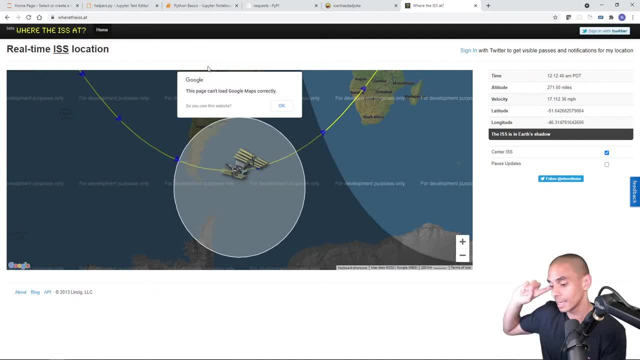 comes to apis. if you wanted to access the twitter api, if you wanted to access the um quandle api for finance data, if you wanted to look at um, the reddit api, there's so many apis that you can start messing around with. all right, we're getting a little too ahead of ourselves what we need to do. 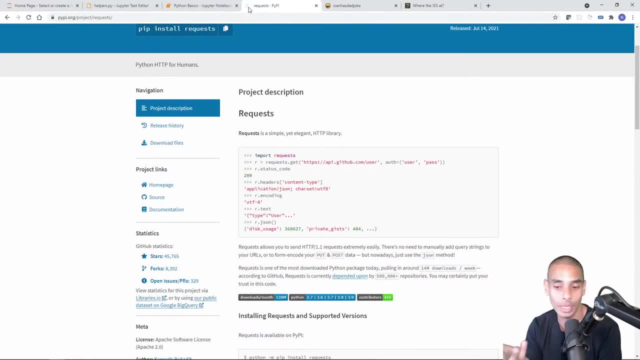 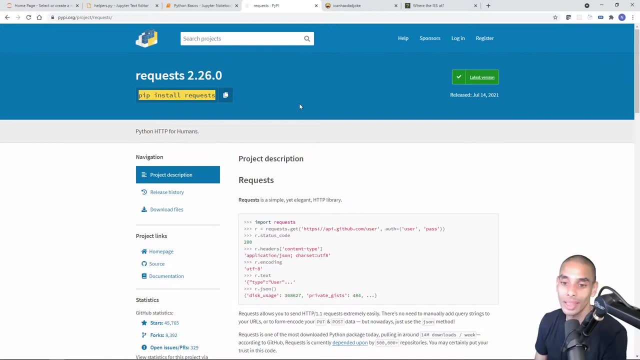 is we actually need to start using the request library to be able to call these apis, and it just so happens that it actually tells you how you can install the request package into your environment in order to do that. so, rather than importing like we did over here, what we actually need to do is: 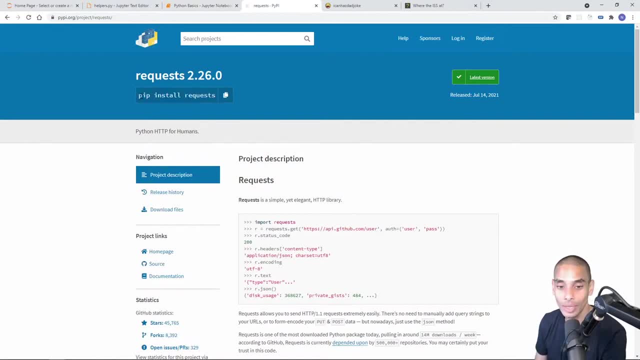 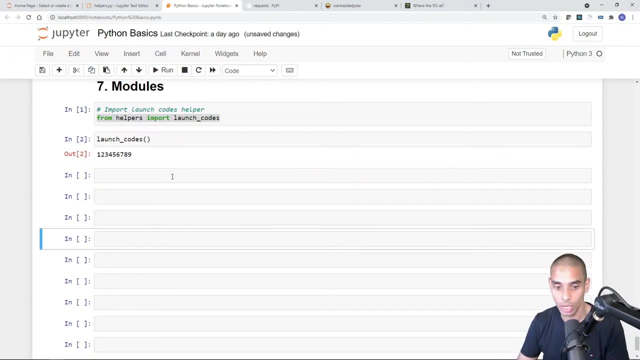 first up, we need to install requests, and in order to do that, we can use pip install requests inside jupyter notebook. but before we do that, let's add a new markdown section, because we want our code to be documented and structured. so we're going to create a new cell and we're going to convert it into a 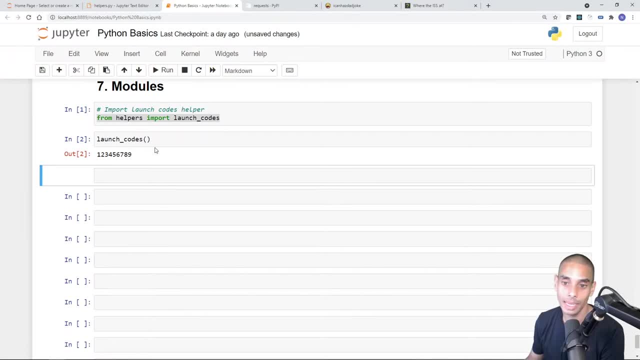 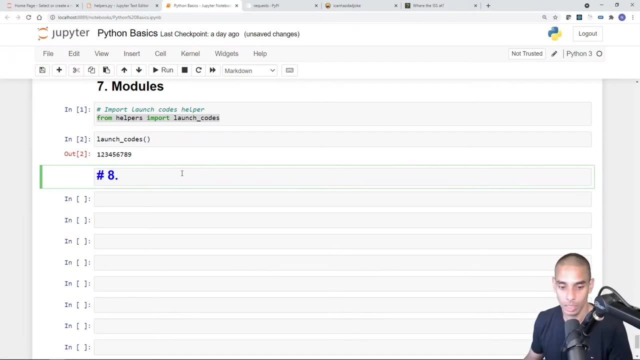 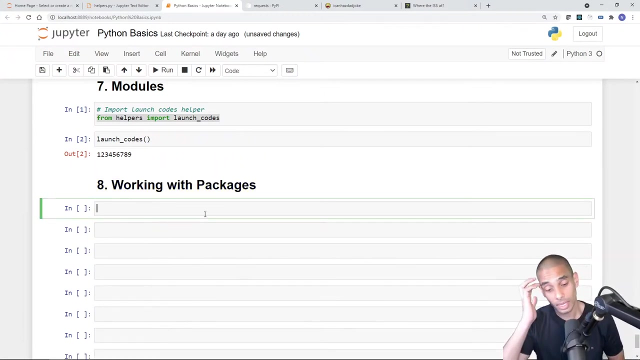 markdown cell, so i'm going to step out of it. hit markdown, then we're going to add a pound symbol and we're going to call this: uh, what are we calling it? let's just call it working with packages. okay, then the next thing that we need to do is actually go on ahead and install. 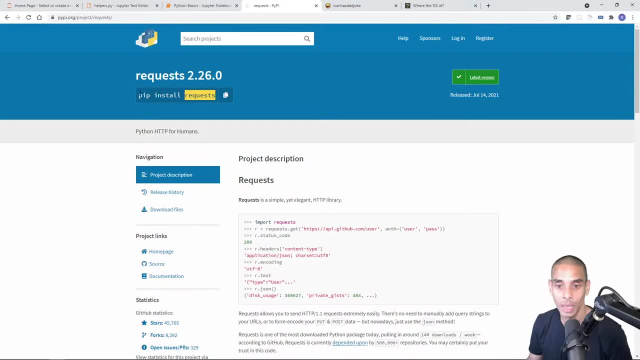 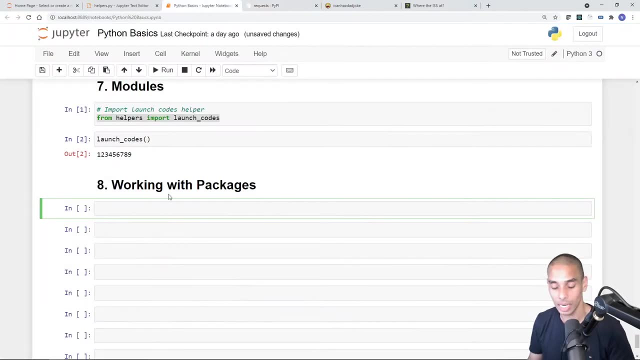 the request library or the request package that we saw from up here. so this method over here, or this little uh bit of string that we can actually copy, so it's pip install requests. we let's actually write ourselves, so we can write pip install requests. and as of right now, if i actually 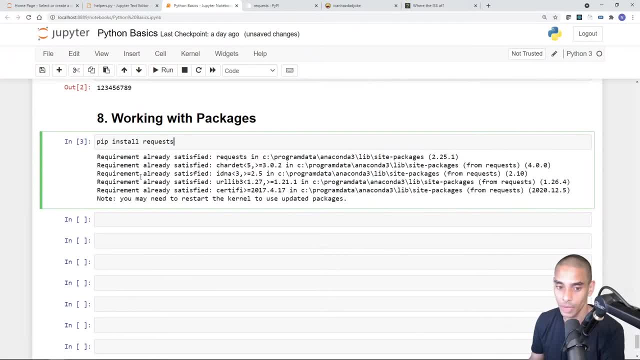 go and run this, this is going to throw- it should throw- a bunch of errors. oh, it doesn't look. looks like we do that without. what you should actually do is add an exclamation mark before this to indicate that you want to run this from a command prompt. so if i go and run this now shouldn't throw. 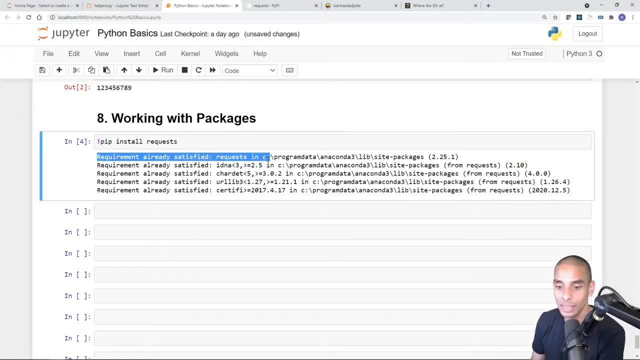 too many errors? all right, so you can see that it's saying requirement or a command prompt and that's okay, we've got that right there. so now if we run this, we can see that we've got this line here. and if we run this now we can see that we've actually got a request ready. 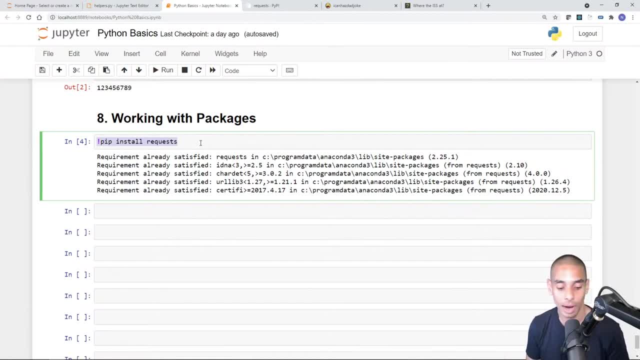 satisfied requests in blah blah, blah, blah. so this line over here is actually going to go on ahead and install that package into the environment that our jupyter notebook is currently running from. so you can see we're currently running from python 3, so that's the environment. 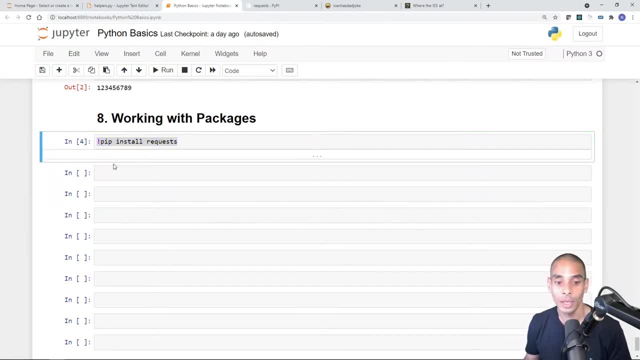 now by running exclamation mark pip install requests. we've actually gone and made this available. now, if you want to see all the packages that you've got available in your current environment, you can act. oh, this is actually something i should show you as well, so see how we've gotten. 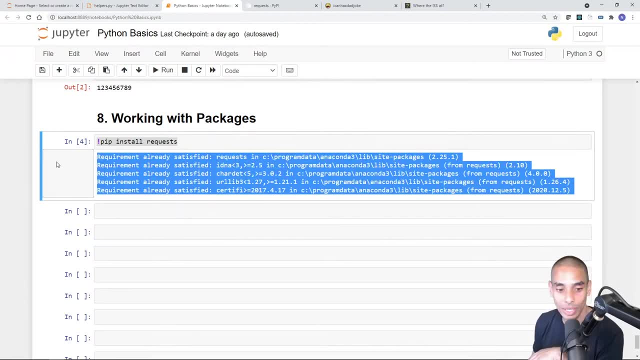 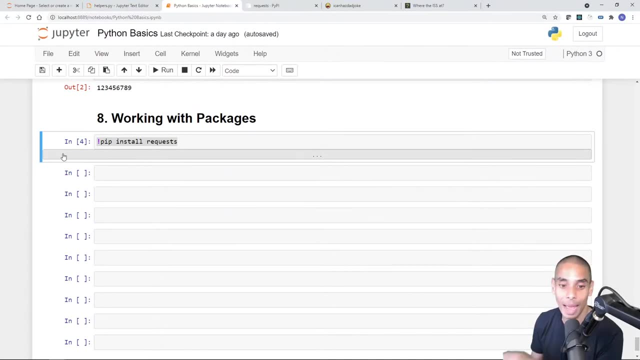 got this big block of text here, right? if we actually wanted to hide that, we can actually select this box over there, so you can see that right over there and this elect actually allows you to hide that output. another thing that you might want to do as well is say you want to get. 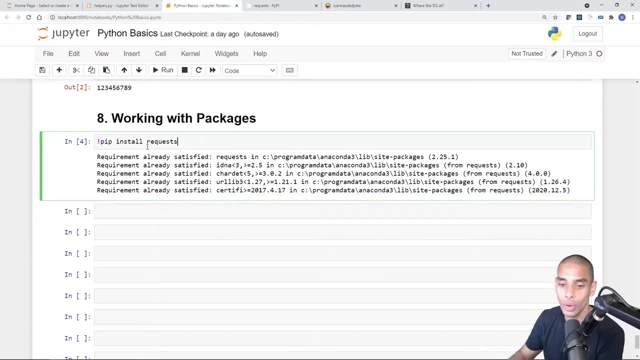 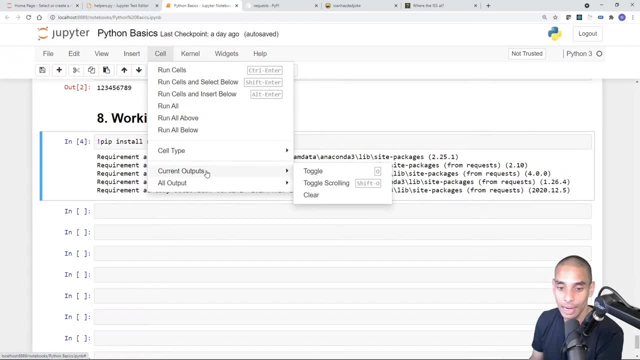 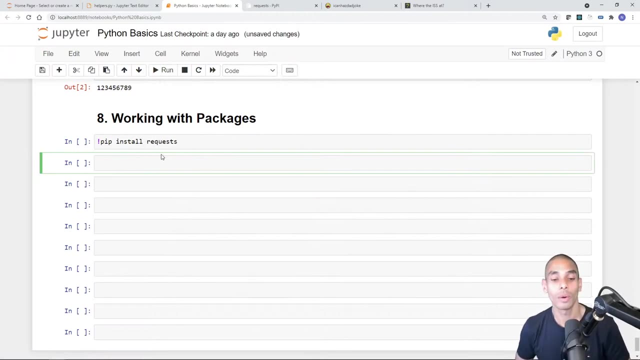 rid of this. so you still want the code cell to have run, but you don't want to see all of this junk over here. what we can actually do is hit cell from our menu bar up here and then go to current output and then go to clear, and that's going to get rid of that stuff down there. now what we can. 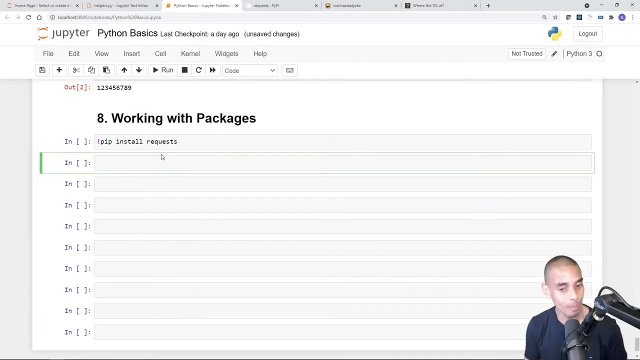 also do, or what we should be doing next is actually importing requests. so so far, we've installed it. oh wait, i was going to show you how to see all the different libraries or packages. so in order to see all the different packages that you've got installed in your current environment, you can hit 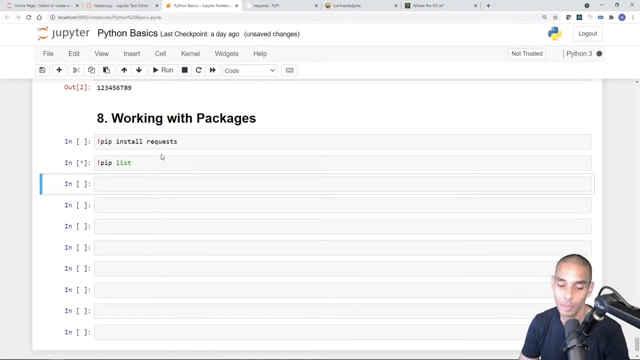 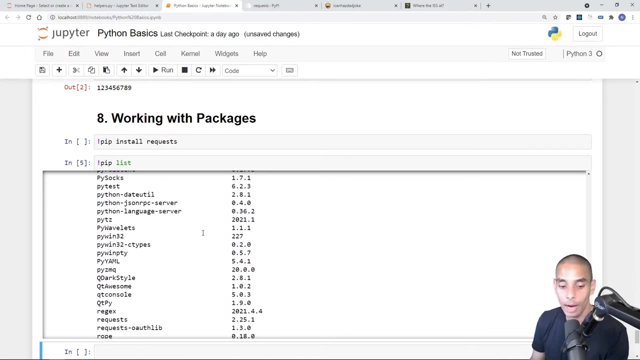 exclamation mark: pip list, and this is going to list all of the different packages that you've currently got in your current environment, so you can hit this and then we can go ahead and hit inside of your environment. now your environment might look a little bit different to this in. 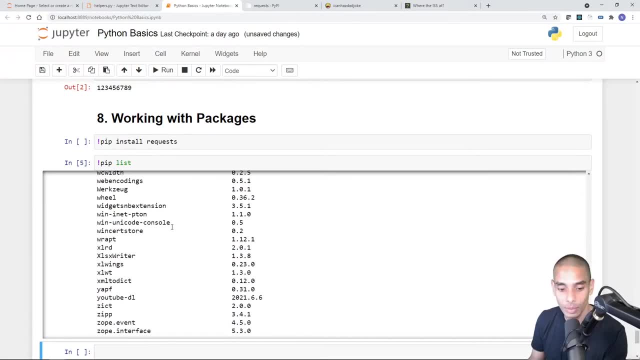 terms of what packages you've got available, because i've been installing a bunch of stuff this week, but ideally you should see all of the different packages that you've got available in your environment. you will also see the package name plus the version that is currently installed. 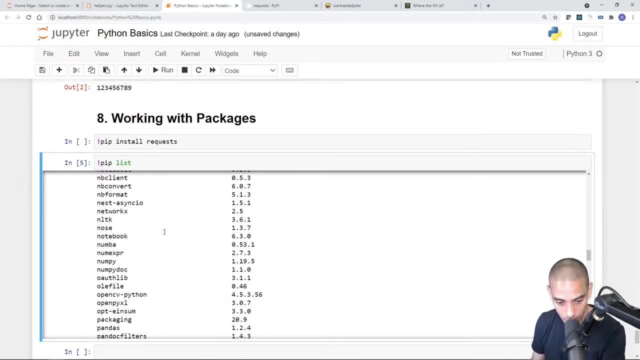 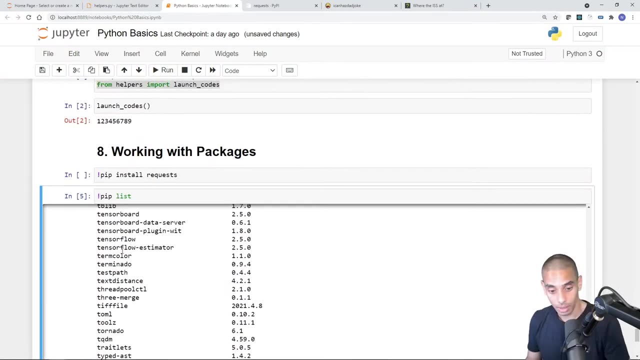 so if we go to, and what did we just installed requests. where are you somewhere down here? oh, my alphabet's not requests. all right, so you can see that we've got currently got requests and we've got version 2.25.1 currently installed. all righty, what are we going to do now? the next: 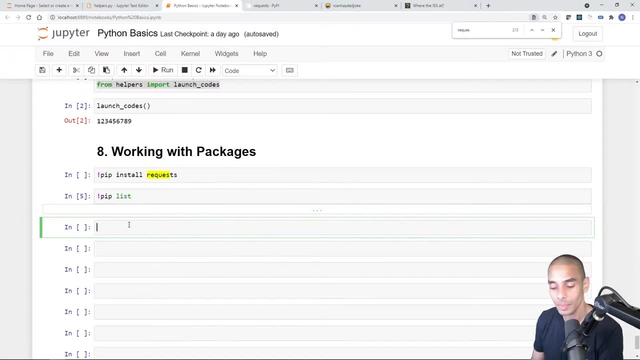 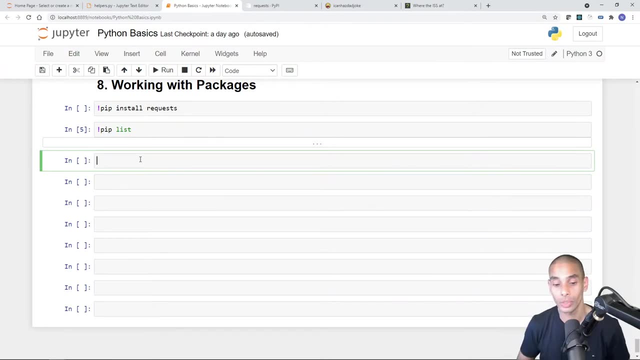 thing that we need to do- and again we're going to toggle this so we can hide it- the next thing that we're going to do is actually import requests. so so far we've installed it, but we haven't brought it into our notebook. so we need to bring it into our notebook so to do that, we can import requests. 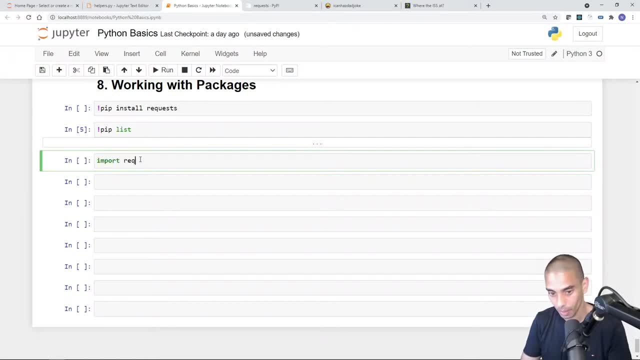 so i just need to type in import requests and again there's a whole heap of different packages that are out there. so again, i'm just showing you one. there's a ton that are out there that you might choose to work with. if you want to see some other examples, do check out some of the other. 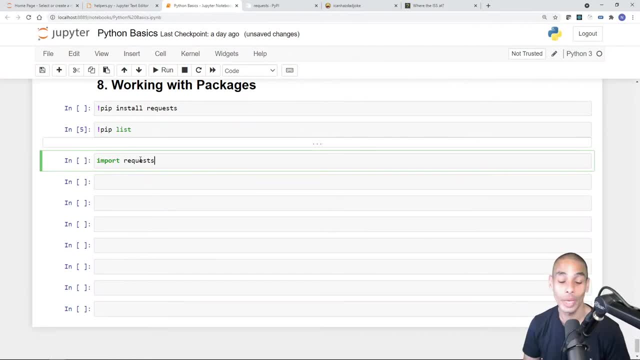 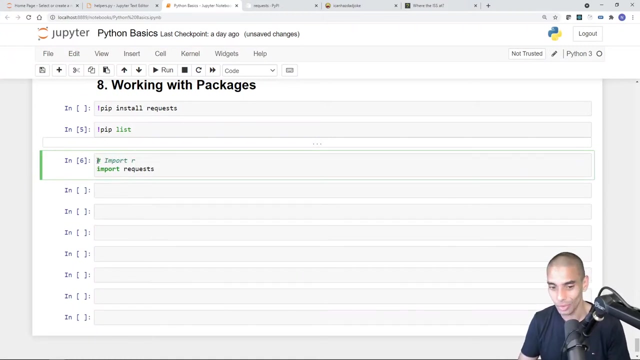 videos on the channel. there's a huge number where we go and use a bunch of different libraries and specifically different packages. so i am going to hit shift, enter to import requests. so now we've got requests inside of our notebook. now let's add in some commentary, so we're importing. it's a little redundant here, but 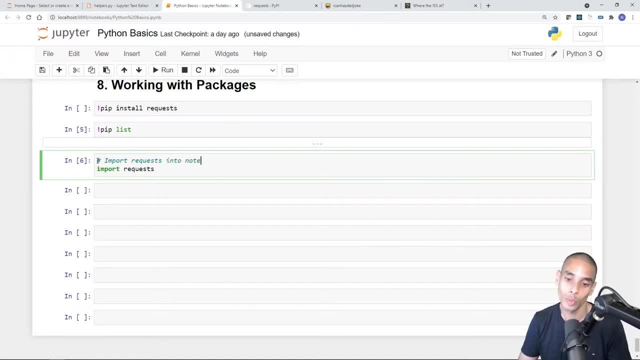 i'm just being pedantic. import requests into notebook, then the let's actually take a look at what we've got from requests. so if i type in requests dot, this allows us to see all the different methods, classes and functions that we've actually got available for our request api. 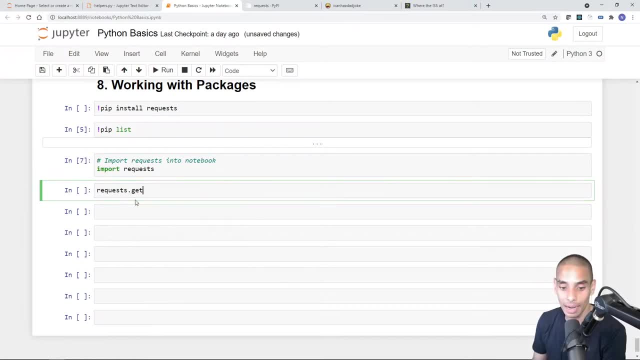 now probably the most important one is going to be this get method. so requestget actually allows us to make a get http request to a specific api. so i'm probably not going to go into too much detail about apis, but you have these different things called, or different. 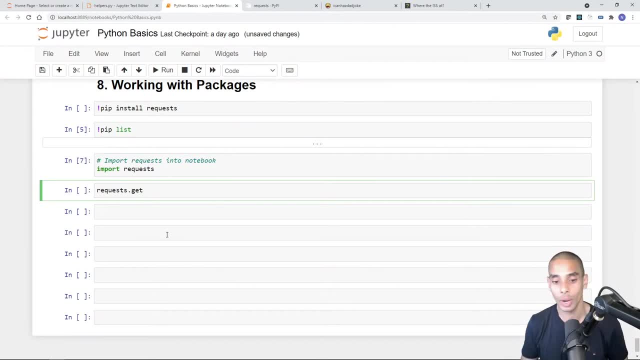 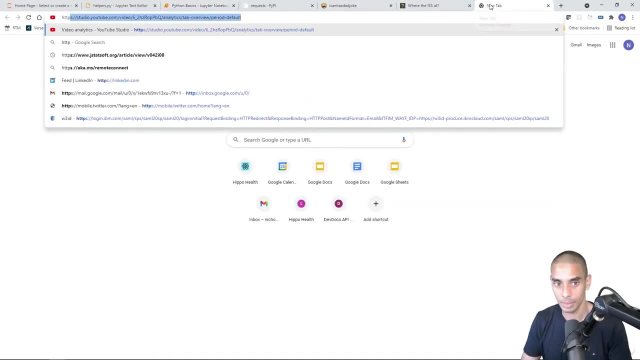 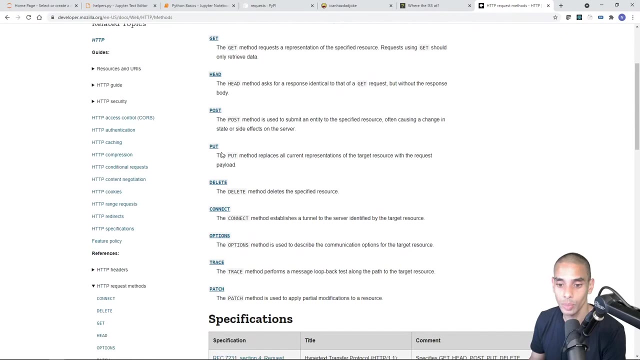 types of methods to call an api. so some of the most common ones are: get put delete. i think there's an update as well. let's actually take a look. so http methods or http request methods, so there you have: get post put delete. connect or patch was the one that i was looking at, rather than update. so 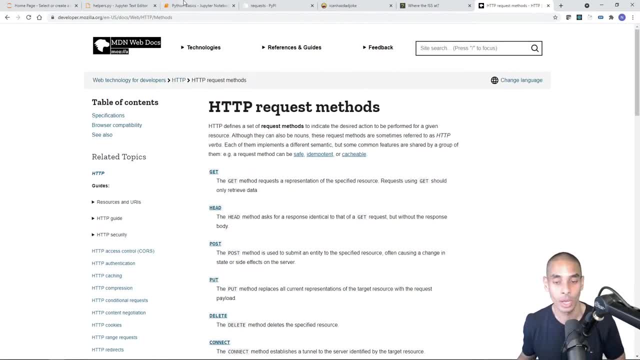 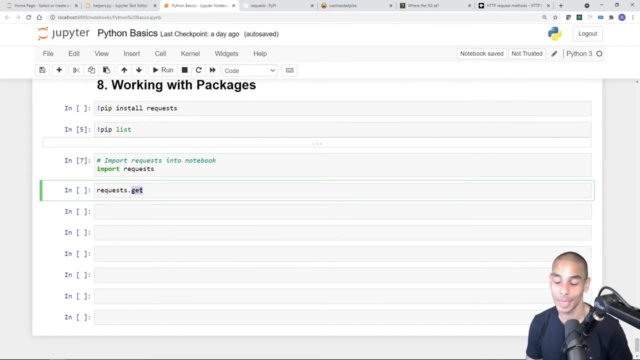 again. there's a whole bunch of different types and i'll make this link available in the description. we are going to be using the get request method to be able to hit our- i has a dad joke- api and our web where the s iss at, api, where the iss at. sorry, i couldn't help myself there, all right, so. 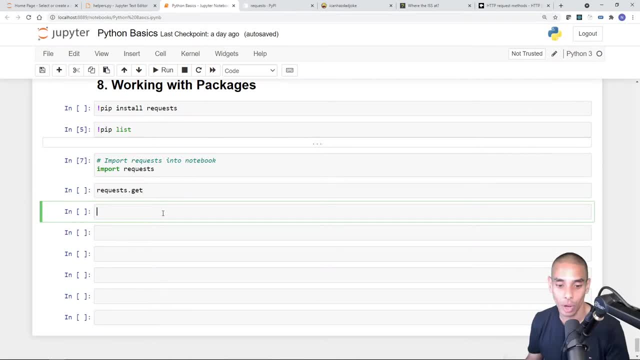 now what we're going to do is: let's set up some variables to hold our apis. oh, we haven't actually taken a look at our api, so let's go ahead and hit our api. and let's go ahead and hit our api and let's go ahead and hit our get function. yet. so if i type in question mark, question mark, because remember. 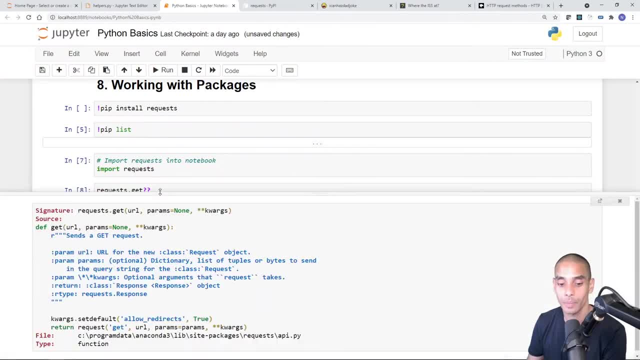 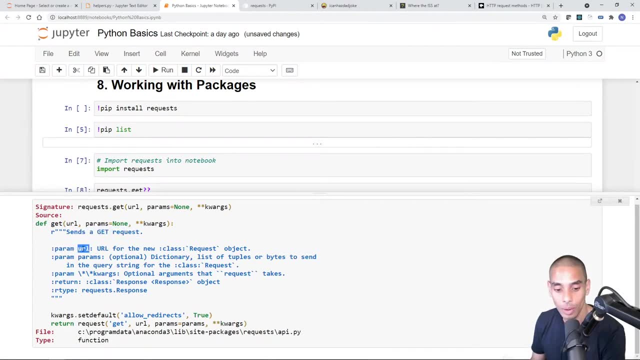 that's how to get the documentation for that method. you can see that this is saying it sends a get request. the parameters that we need to pass through are the url, and then we've got some optional parameters so we can pass through a dictionary, a list of tuples or bytes to send. 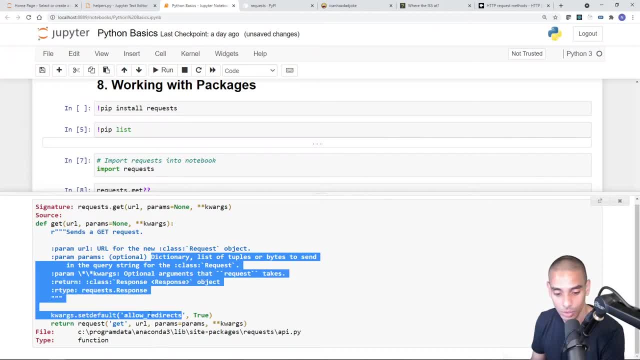 in the query string. we're not going to do too much on that. we can do a bunch of additional stuff, but the main thing that you need to know is that it is expecting a url. it's also expecting some parameters and by default it's set to none, so we don't need to pass those through and it's. 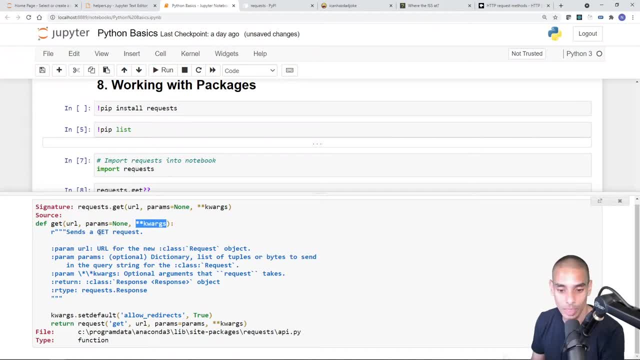 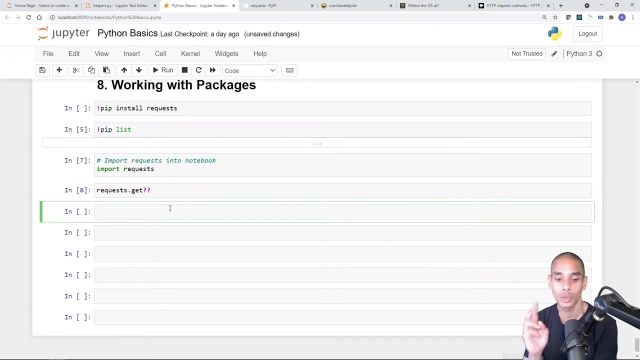 also expecting some keyword arguments, which again are optional in this particular case. so that's sort of how to read documentation. now what we're going to do first up is we're going to set up two variables for our url. so remember we're going to be doing one for i can- has dad joke that api and 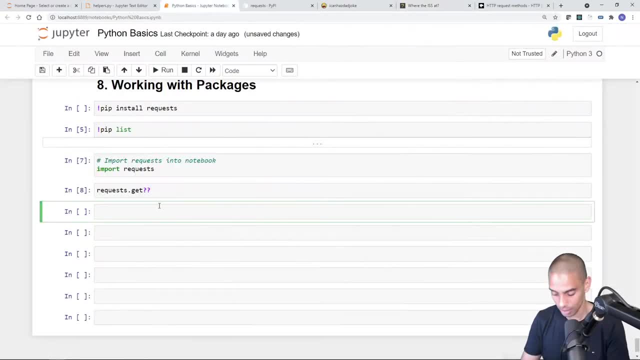 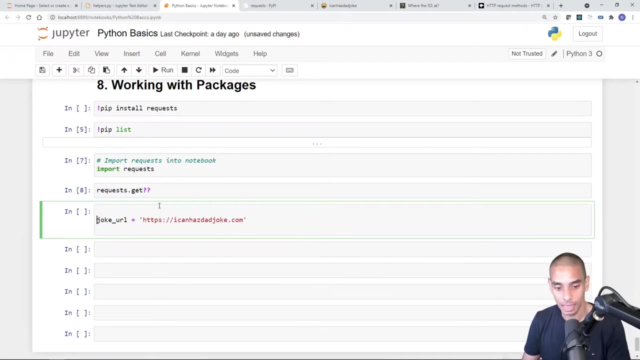 where the iss at. so let's do those. so we are going to create one for the joke url and we're going to set that equal to http. i can has dad joke dot com. i think that's the url, and then let's add a comment. so this is i can. 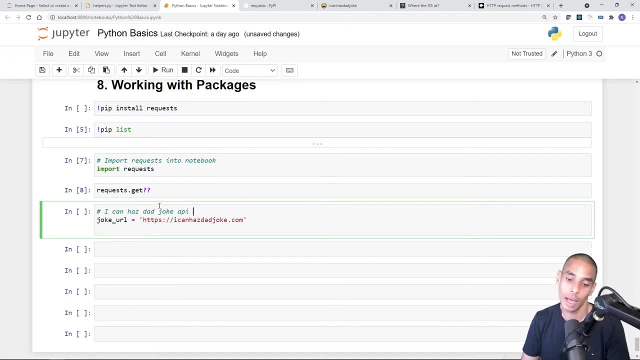 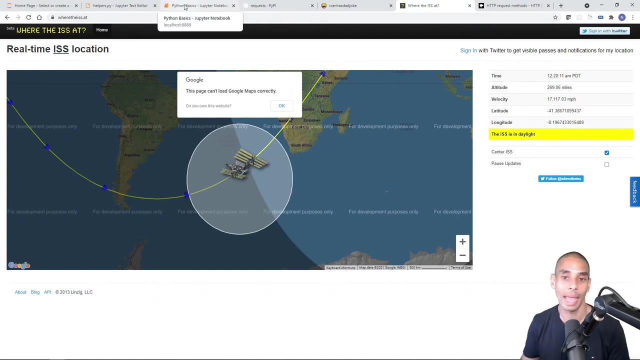 has dad joke: api endpoint. if you hear anybody refer to an api or an api endpoint, the endpoint is really just the url that you need to be hitting, so it's not always the case that the base url is going to be the api endpoint. so in this case, 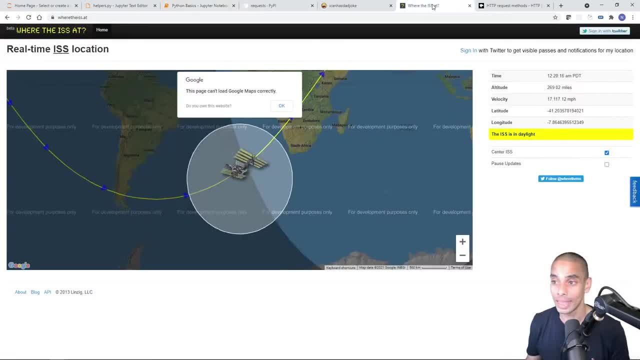 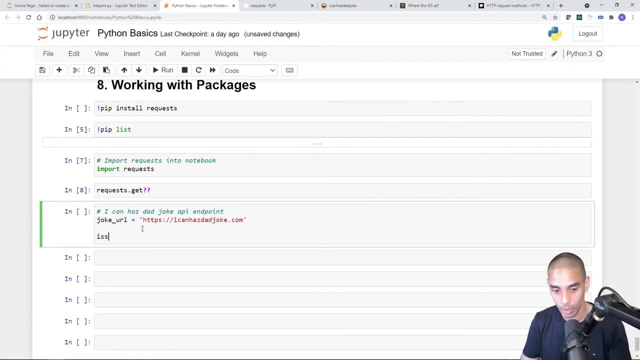 you'll actually see so when i show you the api for where the iss at, it's going to be different to just where the issat, so let's create our iss url and that one is https colon. forward slash. forward slash api. dot where the iss at or dot at forward slash v1. forward slash satellite. 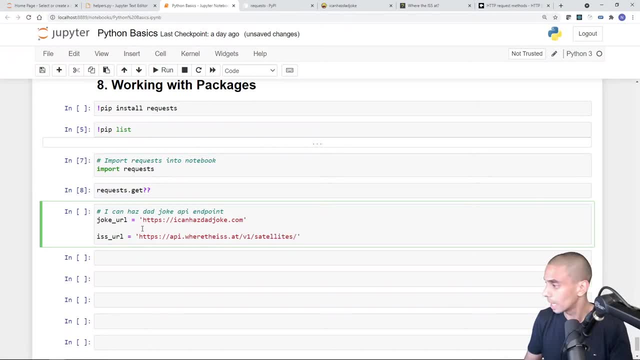 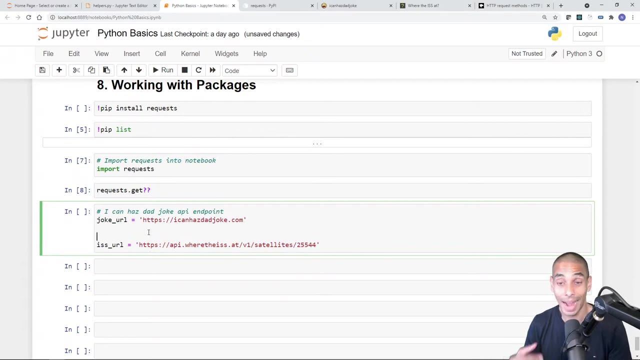 satellites, satellites forward, slash, slash two, five, five, four, four. so this is uniquely different to the icon has dad joke api. but it's also super different to where the issat. so this is a specific url that i went and found that actually gives us the specific details for just the iss. so this is the iss api endpoint. 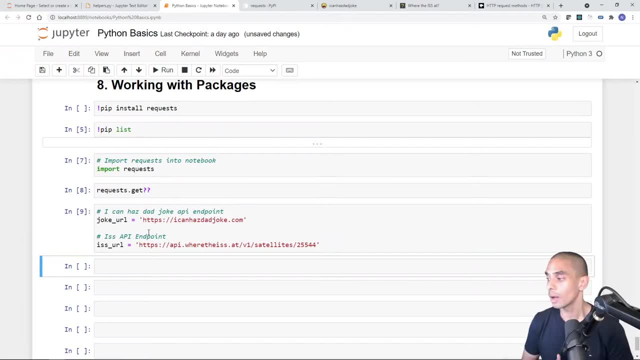 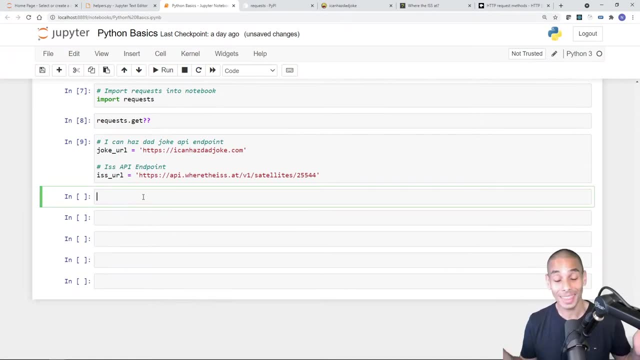 cool, all, right now we need to go on ahead and make our requests. so let's go on ahead and do this. so we are going to, first up, create a variable, and a key thing to note is that right now, we are currently using a new package, so this is completely new. we haven't covered packages before. 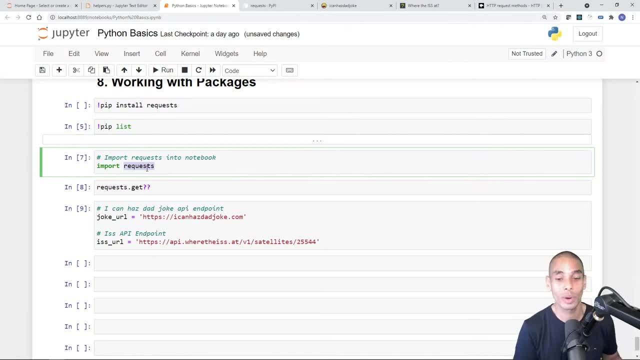 but this extends out. so a good process whenever you're using a new package is to learn how to install it, learn how to import it and then learn the core functions, methods and classes that are available within that package- in this case, the most popular one inside of the request package. 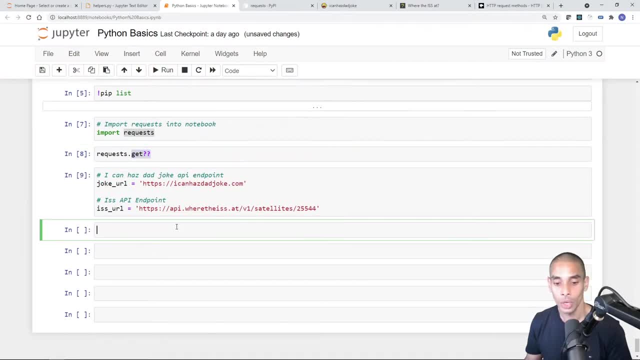 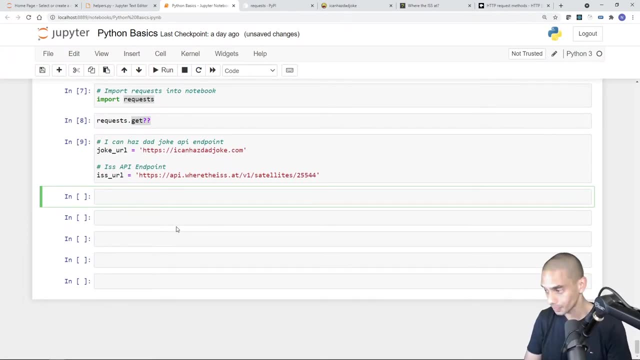 is going to be the dot get method, as you can see there, coolio. so what are we doing? we're going to actually make an api call, so we'll first up do the joke url. so to do that, we need to first up set up this thing called headers or a header. so we are going to create a new variable. 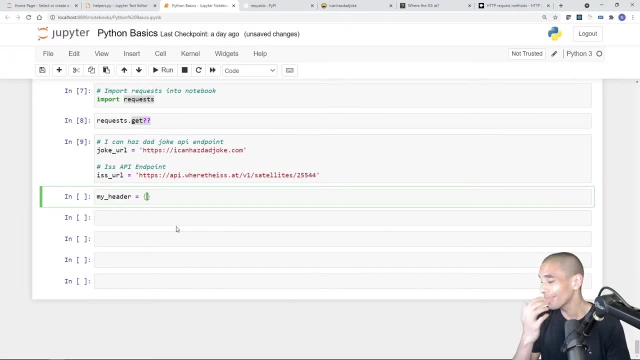 called my header. we're going to set it equal to a dictionary and think of a header as like some metadata that we send with our api call. so sometimes you might send through your authentication tokens. if you have a protected api, you might also specify what type of data you want back. you might also 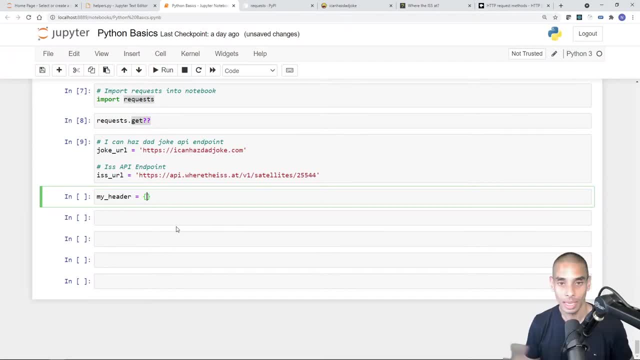 specify what type of data you're sending as part of the api call. keep in mind there's a ton of stuff you can do with apis. that's probably a topic for a whole nother video that we might need to make now. let me know if you want to see a full video on apis, and then what we're going to do is we're. 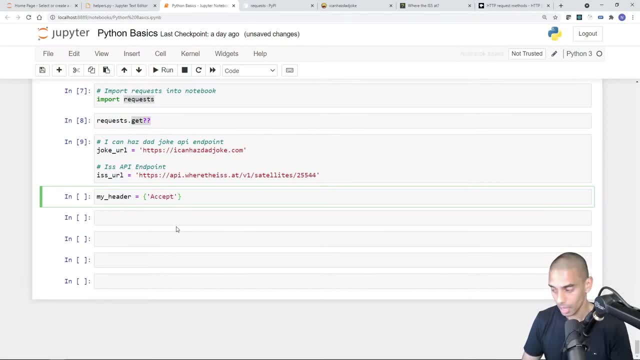 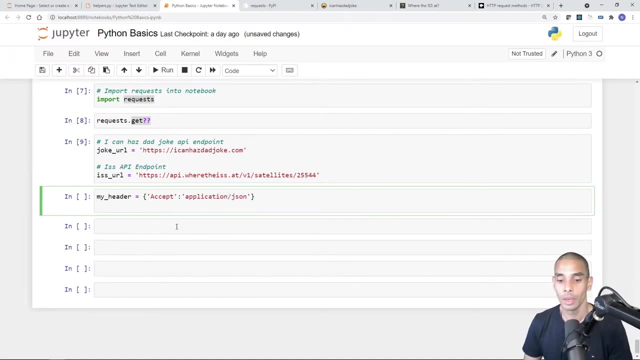 going to say that we want to accept, and we are going to accept json back as our response application for json. cool, now what we want to do is actually make our api call. so let's actually specify: so this is going to be our api call. so we're going to set up our api call and we're going to 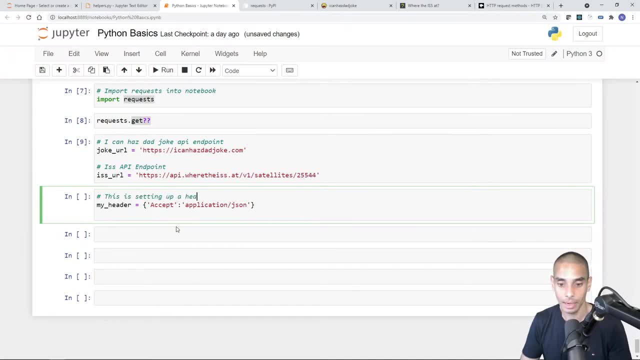 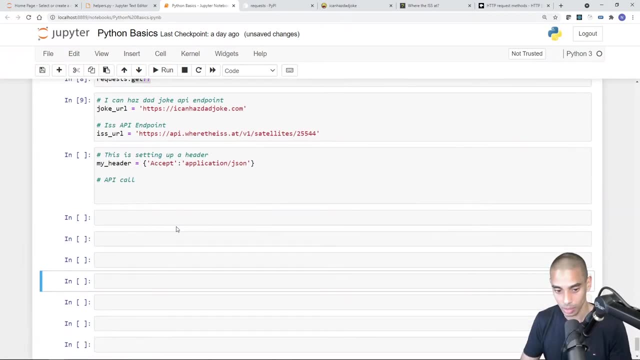 do this. so this is setting up a header and then we can actually make our api call. api call: let's add in some more cells below so we can center that up. and then in order to make our api call, so we first up need to pass through our url and then we're going to pass through. 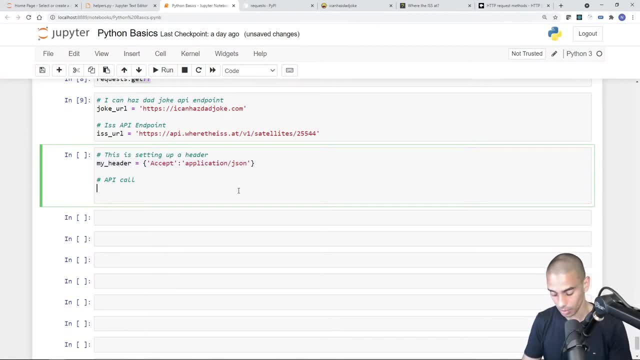 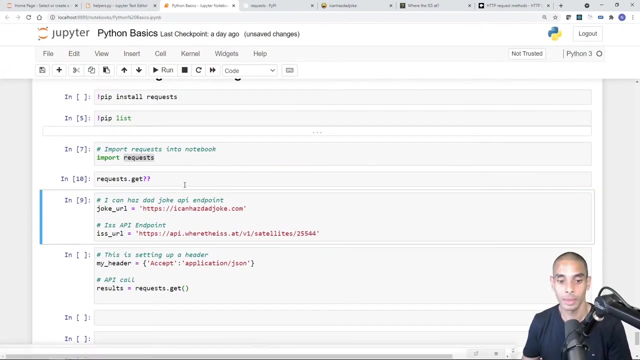 our header. so let's do this. so i'm going to pass through, uh, results. that's actually yeah. so let's store our results inside of variable called results and we're going to call requests. so all right, and then the first thing that we want to do is pass through our url, because, remember, 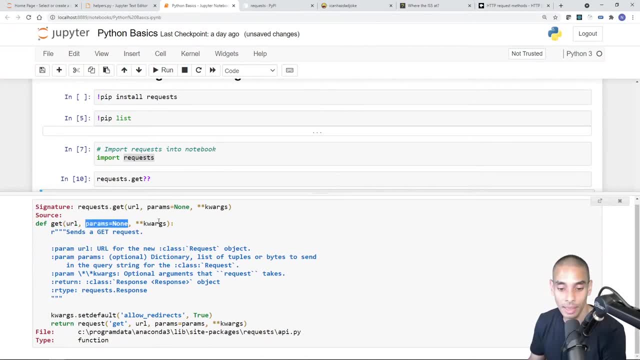 our request. api is expecting our url first, and then it's expecting some parameters and some keyword parameters- in this case, our params is set to none- and our keyword arguments. there's a whole bunch of them if you actually take a look at the documentation. so go to requests. 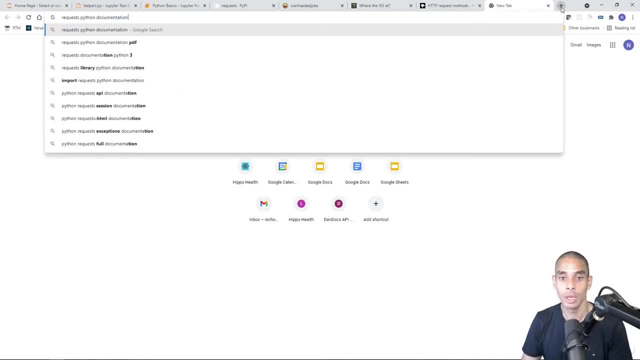 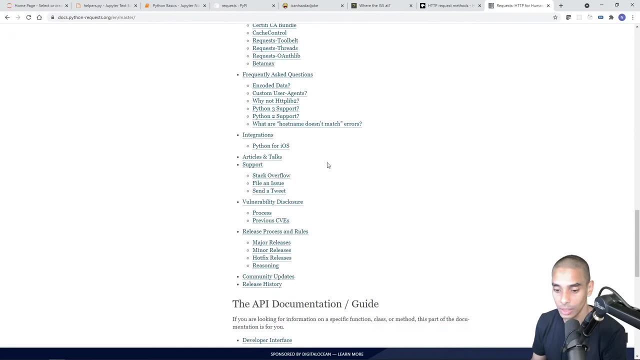 what is that? requests python documentation, chrome, oup. there is a ton of options that work with the request library, So we're going to take it super easy, but there's a ton of information about this. Really really good practice whenever you're dealing with a new. 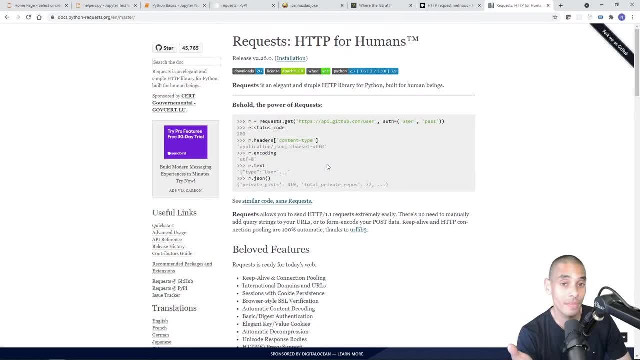 package to actually go on ahead and read the documentation. More often than not, the most popular Python packages are going to have really really good documentation because they're well supported packages. So TensorFlow is a great documentation, Pandas is great documentation, So does NumPy, So does PyTorch. So if you want to play with some of those libraries, 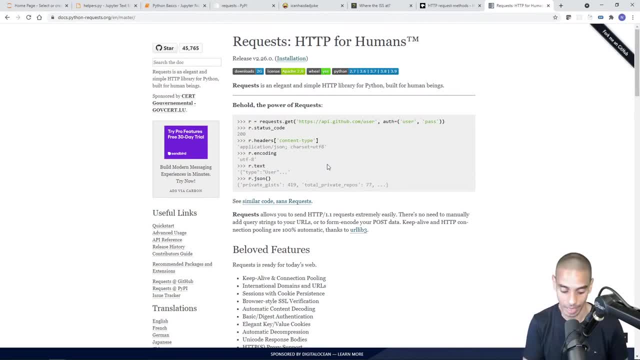 do read the documentation. This is what allows you to transfer from being a junior developer or someone that just tinkers around to being a really, really good developer. Learning how to read documentation is going to make all the difference, So in our particular case, we can. 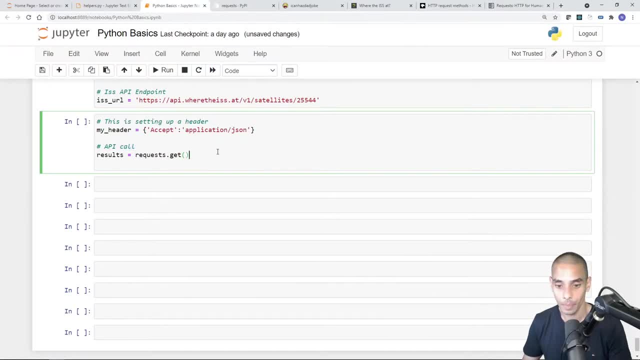 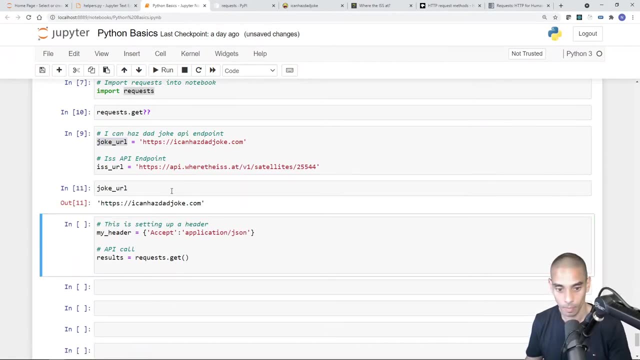 close this down and we are going to pass through our URL first up, which, in this case, is going to be our joke URL, which is just a string. So if I type in joke URL, it's literally just a string that contains our API endpoint. So if we pass through our API endpoint, we're going to see 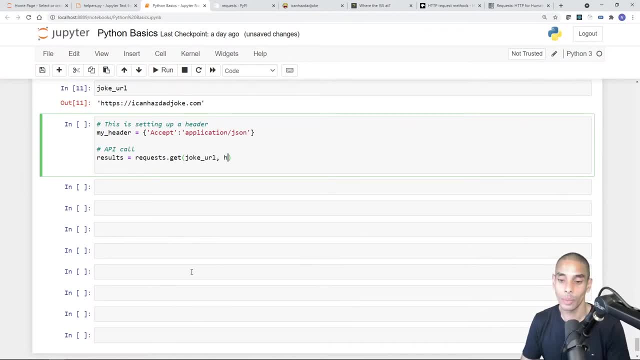 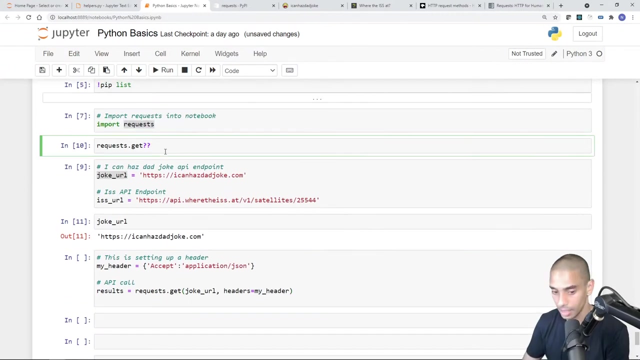 our joke URL And then we need to pass through some keyword parameters. So this particular case, our keyword parameters are going to be our headers. So we type: headers equals my header Right. So remember when we took a look at our documentation. let's run this again. 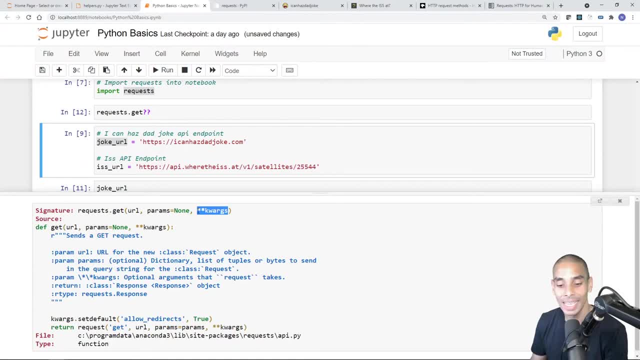 We said that. so this little argument over here basically says that this particular method is going to accept a bunch of different types of keyword arguments. So the star star basically unpacks the argument. So we're going to pass through our joke URL And then we need to pass. 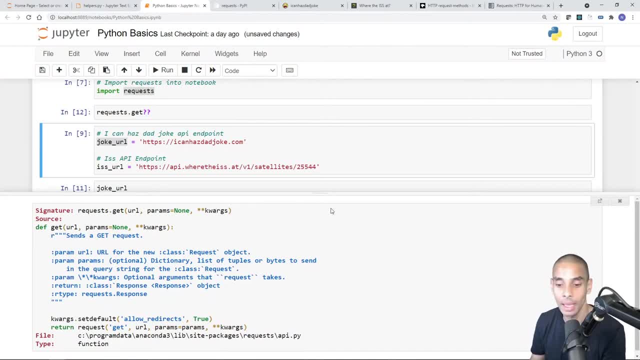 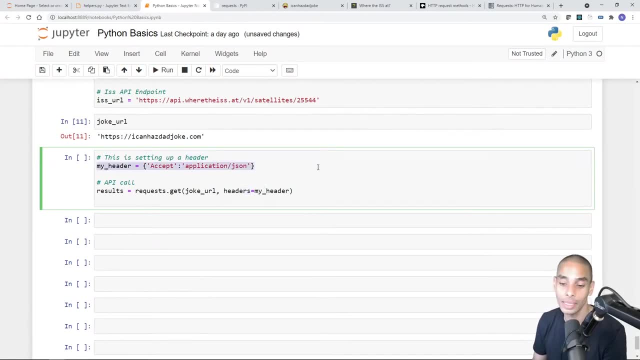 a bunch of keyword arguments, So there's a bunch more than what's specified there. Now, in this particular case, one of our keyword parameters that we can pass through is headers, And this header is allowing us to return back JSON. So you'll see this in a second, So let's take a step. 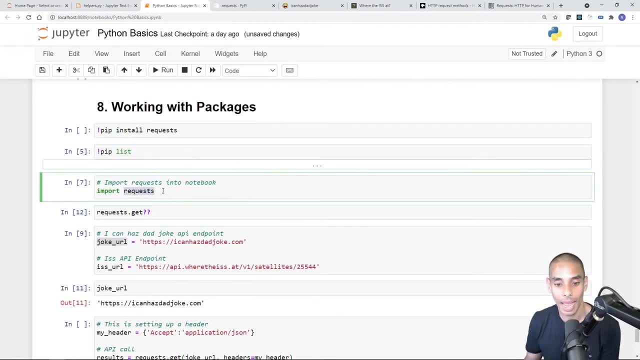 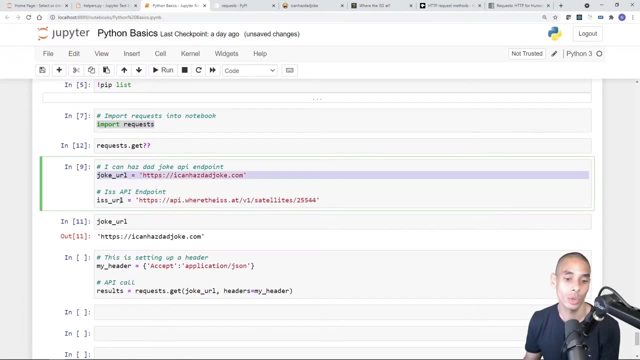 back. So what we've gone and done is we've gone and installed requests, We've gone and imported it. We've then gone and set up two API endpoints- So joke- underscore URL and ISS underscore URL. We've then gone and set up a header And then we've gone and imported it, And then we've gone and set up an. 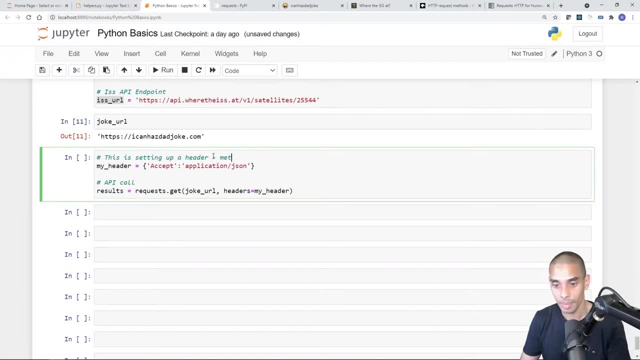 header. And remember a header is like metadata, metadata for your API request, And then we've actually gone and set up our request in this particular case, or our API call. Then that particular line, we've written results equals requests dot get. And remember, there's a bunch. 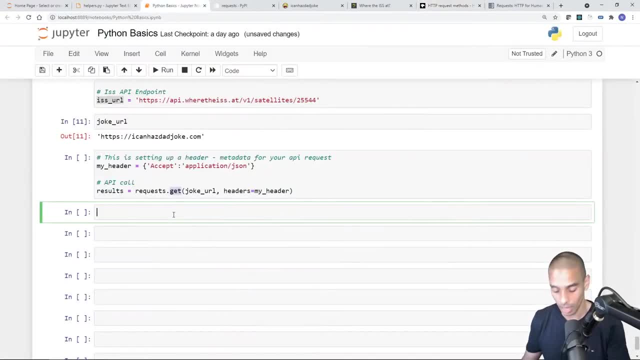 of different HTTP request methods. So if we actually type in requests, dot put, that's another one. request, Dot delete, that's another one. Request, dot patch, that's another one. So again there's a bunch of different types of HTTP request methods that you can make. So more often than not you have to look. 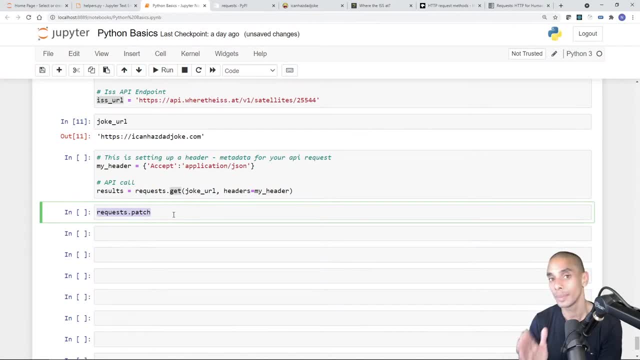 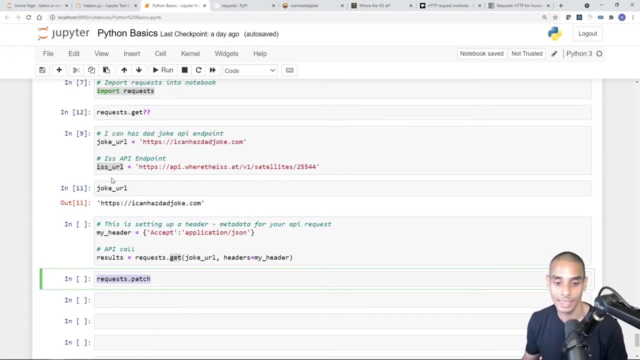 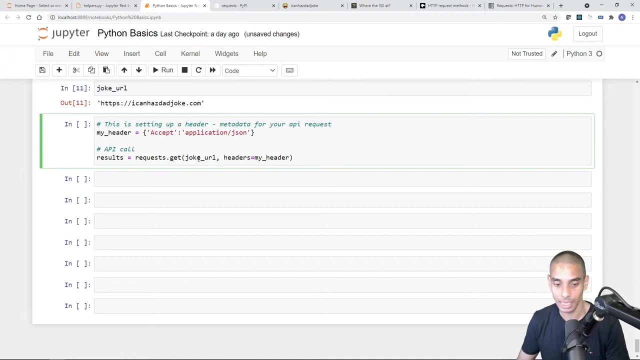 at the API documentation to understand what type of HTTP request methods a particular API can take. In this case, I know that the joke URL and the ISS URL can handle get requests, So we're going to do exactly that. Okay, so we've gone and done this. Let's actually make our API call now. So if we 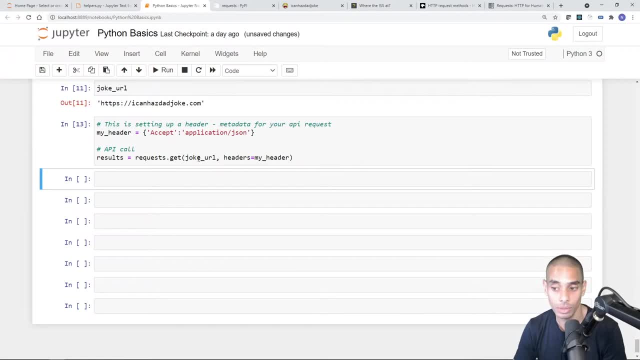 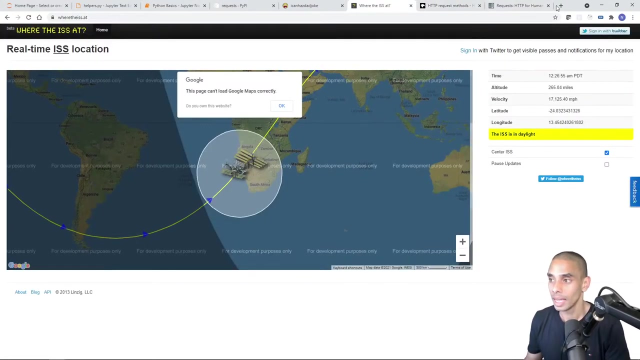 run this cell fingers crossed that looks like it's been successful. So we don't actually know yet. So let's actually deconstruct this. So if we type in results, you can see that we've got a status code return. So if I take a look at HTTP status codes, there are a bunch of different types. 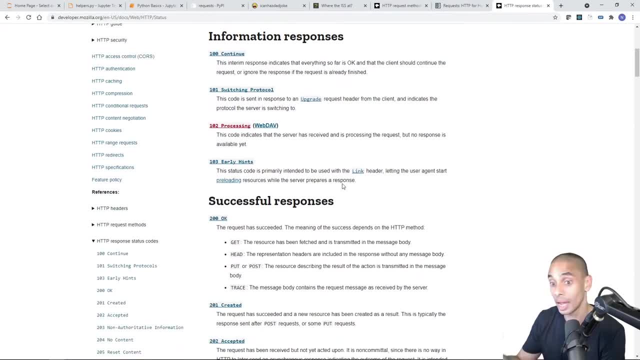 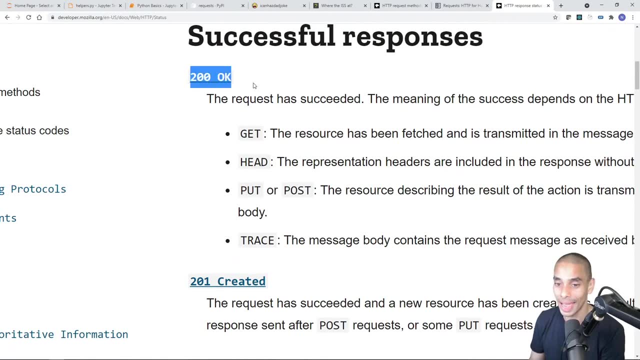 of status codes that you'll get back when you make an API call, In this particular case, a status code of 200, which you can see there- basically means that we're okay. I like how lackluster that is. It's like: yeah, we're okay, we're cool, But it basically means that your API request has been. 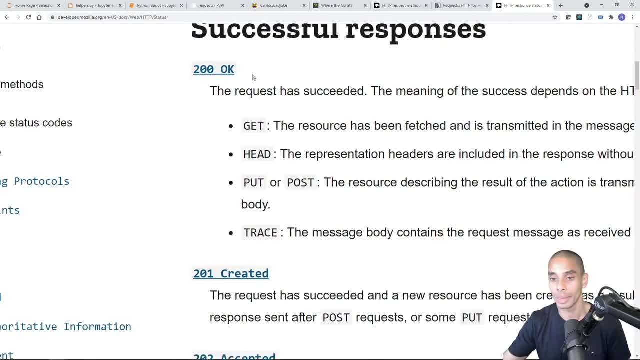 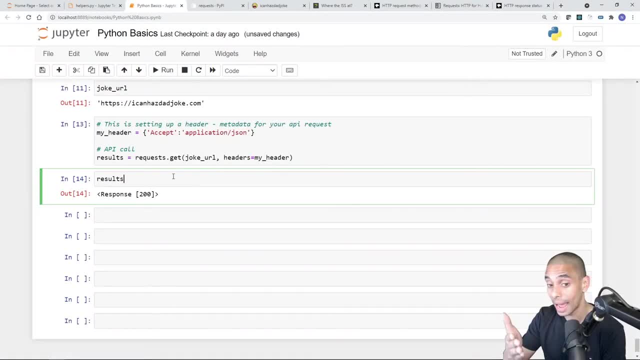 successful. So you don't have any errors. you've actually got something back. Let's zoom out of that. So how do we actually go and see what our API call is actually returned back? Well, we can actually type in dot And we've got a bunch of variables that we can actually return back. So 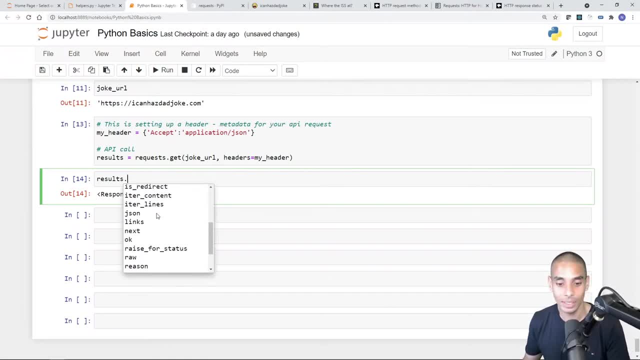 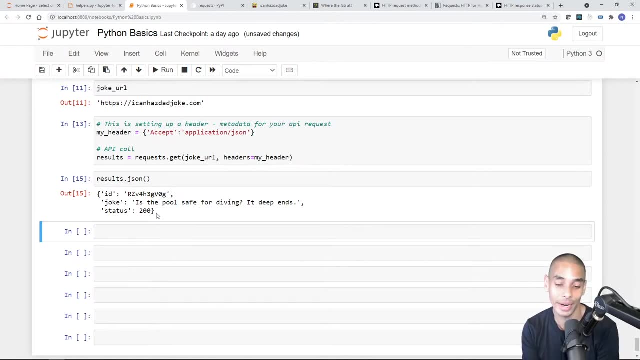 we can actually get back from this. So the one that we're going to take a look at is dot JSON, And so you can see there that what we've actually got back is a dictionary, And in this particular case, our dictionary is represented as JSON. So if we actually store this result inside of a JSON result, 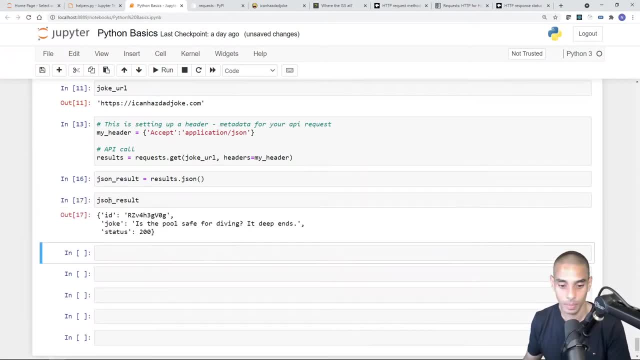 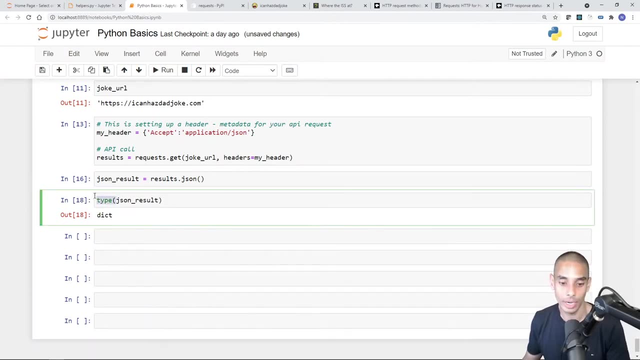 variable, JSON result and if we type in type, you can see it's a dictionary. Cool, So remember: type allows us to check what type our variable is. in this particular case, it's returned dictionary And we've got back. let's actually take a look at our result. So we've got back three. 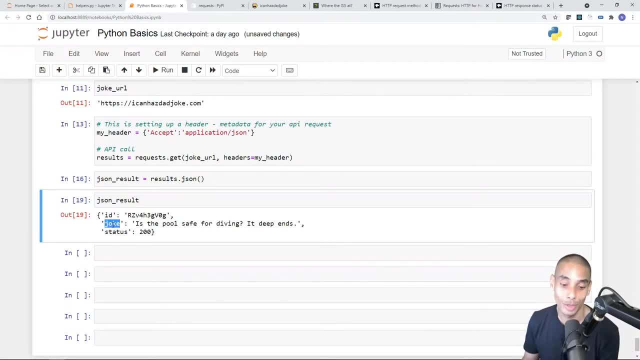 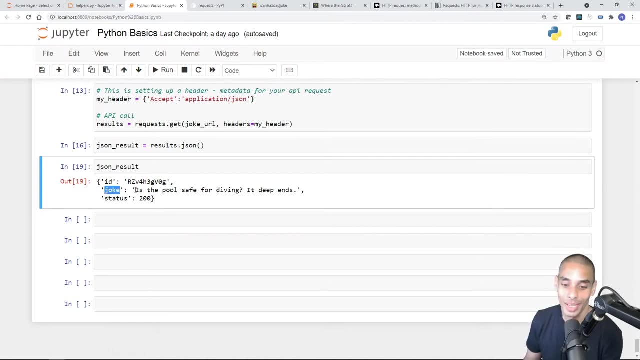 different keys. So we've got back an ID. We've also got back the joke itself And we've got our status code. So this ID is just a unique identifier. This joke is actually our joke, So this is the joke that we've got returned back. So is the pool safe for diving It deep ends? Oh God, that's terrible. 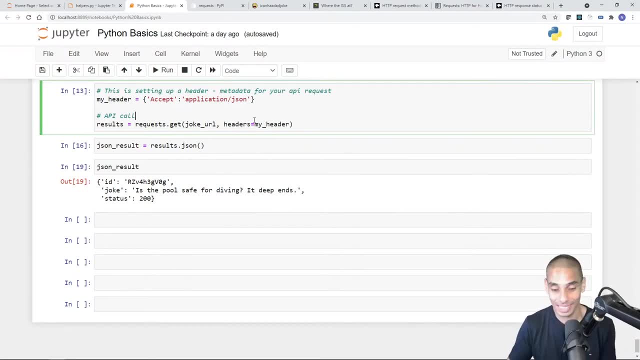 All right, let's do another one. So if we go and run this cell again, it's going to make another API call and return a different day dictionary. Yeah, that joke was terrible. Sorry, guys, My bad. All right, let's run this. 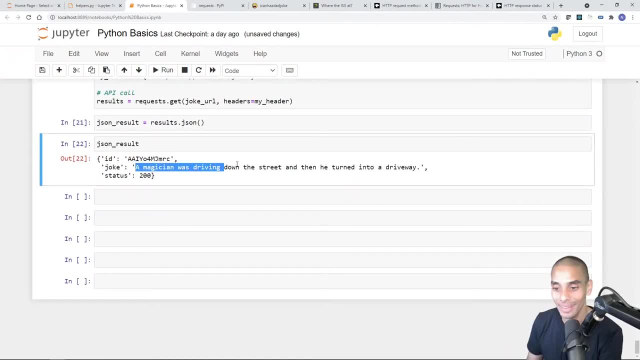 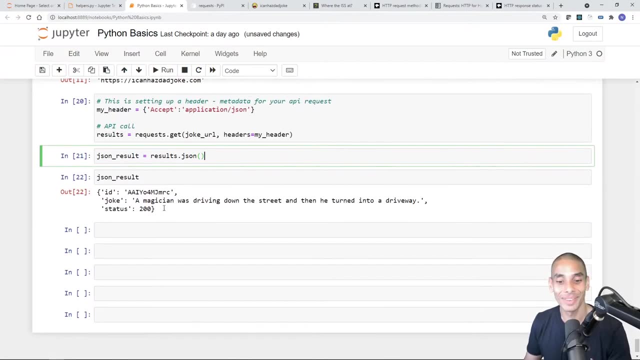 again. All right, what? this is our next joke- that a magician was driving down the street and then he turned into a driver. Oh man, these really are dad jokes. Yeah, I had to bring this one on yet, But you can see there that this is actually making an API call across the internet, keeping you need. 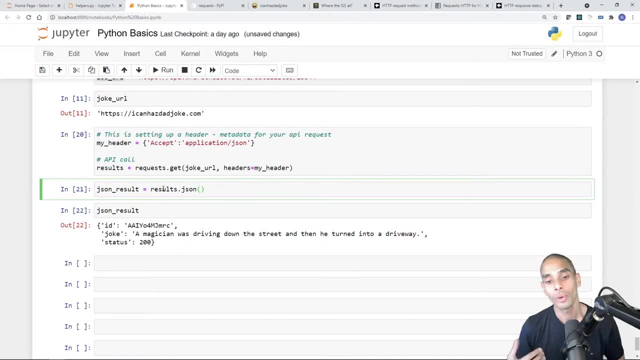 to be accessed or connected to the internet. for this to work, We've gone and made an API call to an endpoint, So this opens up the whole wide world to you. So if you wanted to do stuff with this, you definitely could. Now you're probably thinking: 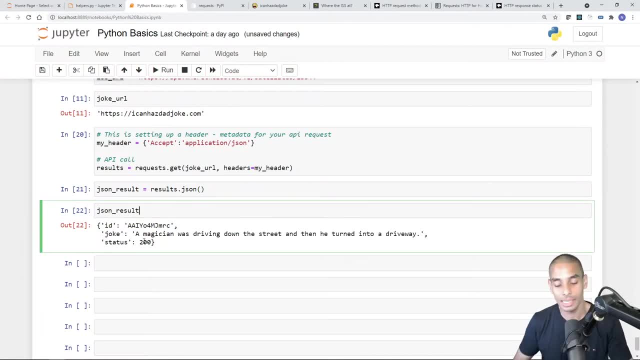 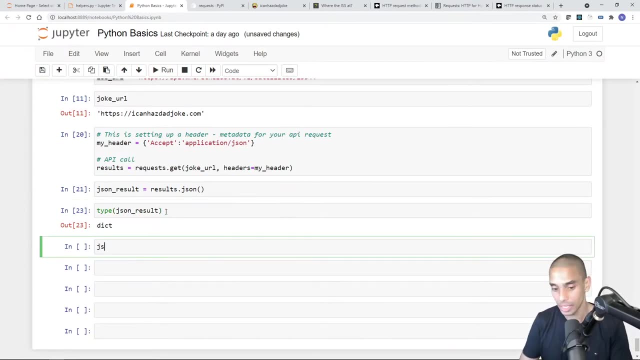 how do I just get this joke right? And again, because this is a dictionary. so we can prove that by typing in, type around a variable. It's a dictionary. So how do we get our data out of a dictionary? So remember, we can access it using the keys, And we've got three keys here, So we've 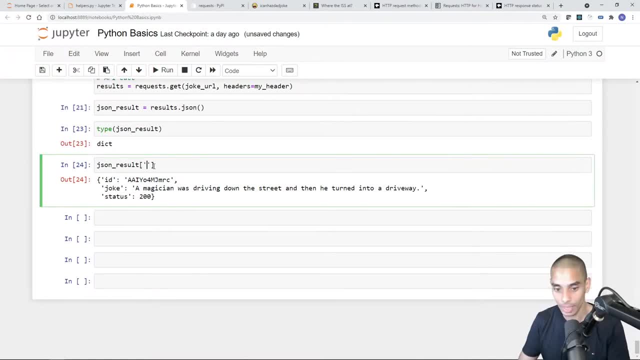 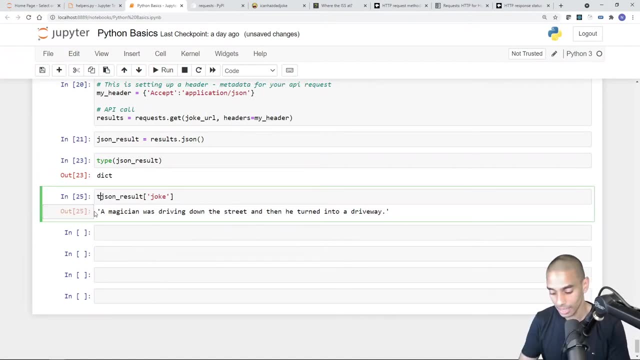 got ID, we've got joke and we've got status. So to get a joke out, we can type in inside a square: that's joke And that brings back our joke as a string. So if we check this type, you can see. 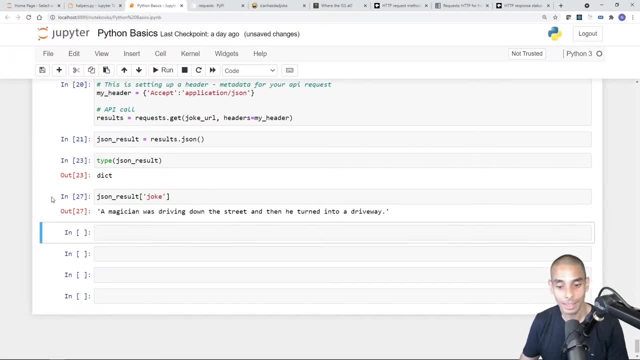 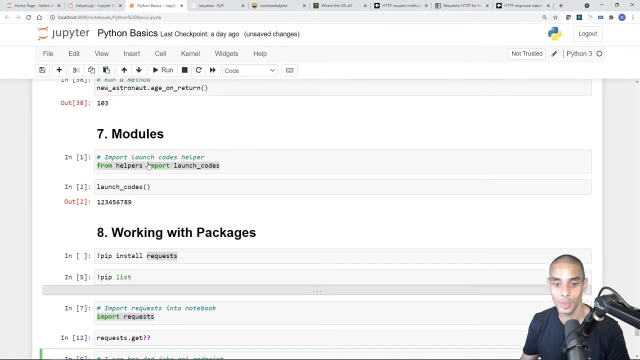 we're getting a string back. Pretty cool, right? So that's API calls now done. Now, what we can also do is we can also make an API call to our ISS API. Remember this one over here. But before we do that, let's actually do a recap. So remember, we've gone through modules so far and we imported. 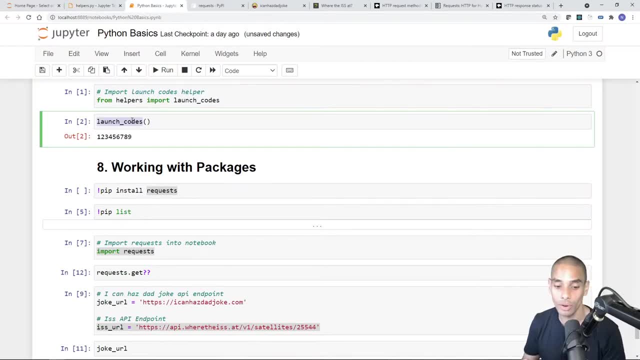 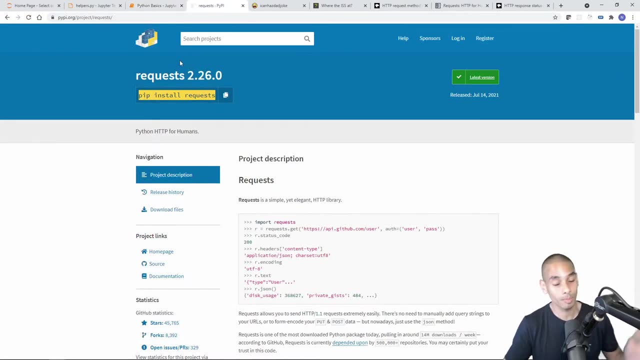 API. We also went and ran a function that we imported from our helpers. We went and installed packages And remember there's a bunch of different packages available from the Python PyPy repository. Remember, this is the collective knowledge of all the different Python developers. 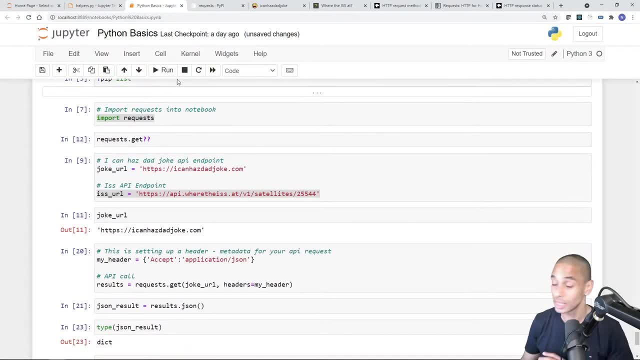 out there. We can also make API calls using specific packages And one of the most popular for that is the request package. To import it. we can type in import requests And then one of the most popular methods which is attached to the requests. 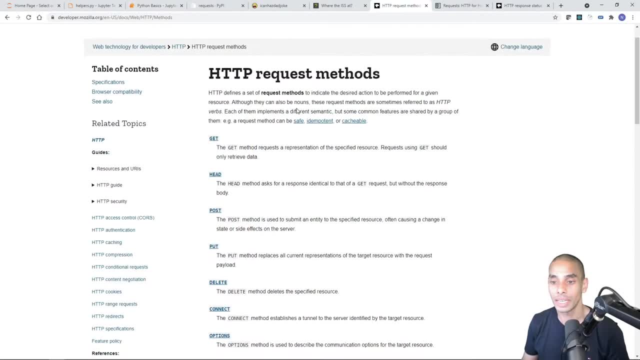 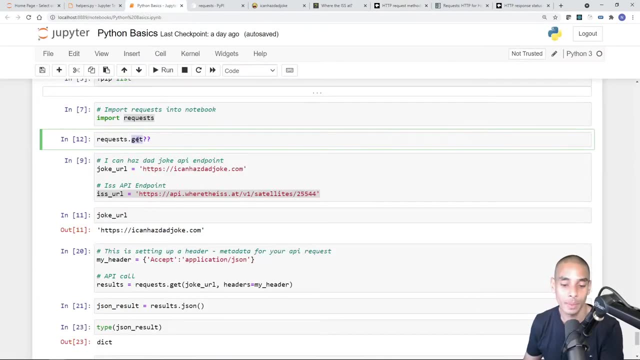 Package is the get method, And remember there's a bunch of different HTTP request methods that are out there in the World Wide Web. In this case, get is one of the most popular ones. Now, in order to make an API call, we can use that method. So requestget, The first parameter that you need to. 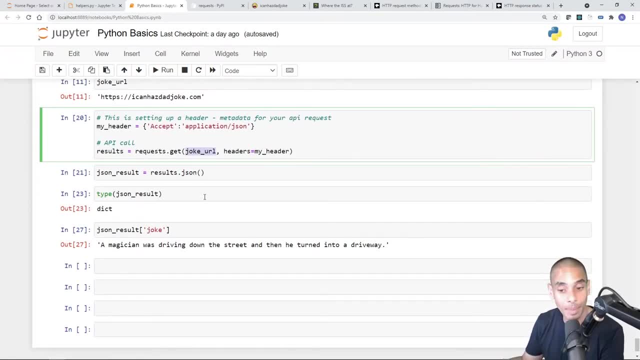 pass through is the URL or the endpoint for the API, And then we can pass through a number of parameters. In this case, we're passing through a header which is saying that we only want to accept JSON back And JSON is just another data format, right? It looks really really similar to a dictionary. It has some 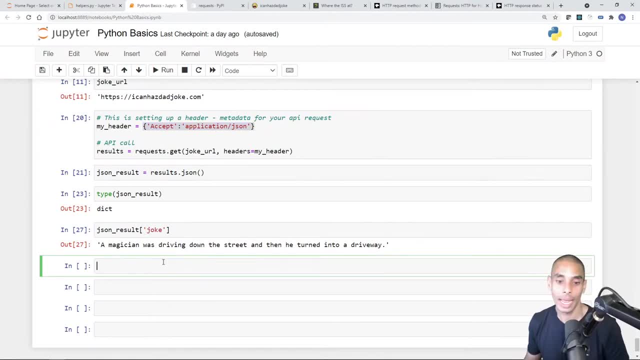 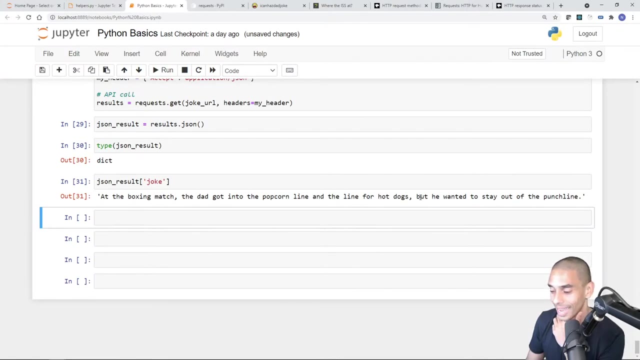 specific properties. We can get into that later. if you want, Let's go on ahead and make another one more joke. I want to see how bad this gets At the boxing match. the dad got into the popcorn line and the line for hot dogs, but he wanted to stay out of the punchline. Oh man, Ouch. Okay, All right. 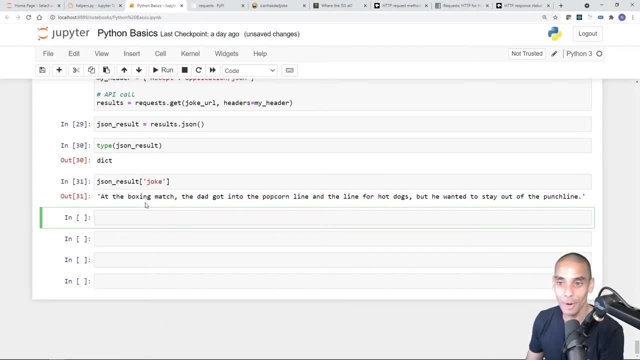 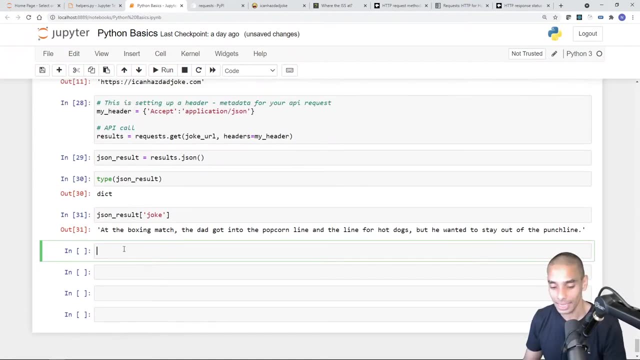 So let's go ahead. Rather than taking a look at any more of the ICANN- Has Dad Joke? API, let's skip on over to the ISS API. So we're going to make an ISS API call now, And this is live tracking, where the ISS is Pretty sick, right. 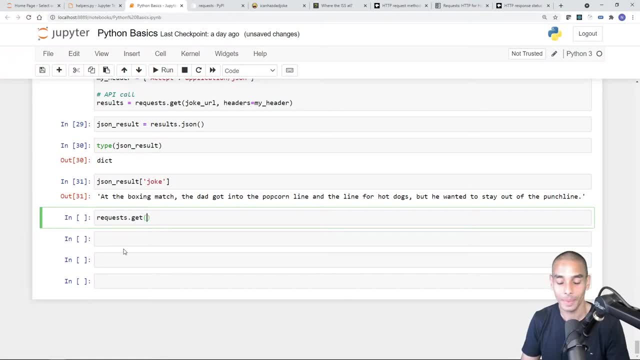 So we can type a requestget And then we're going to pass through our ISS URL. So this up here, ISS URL, And then we're going to pass through some keyword parameters. We just need our headers Headers. Let's make this a little bit more centered. 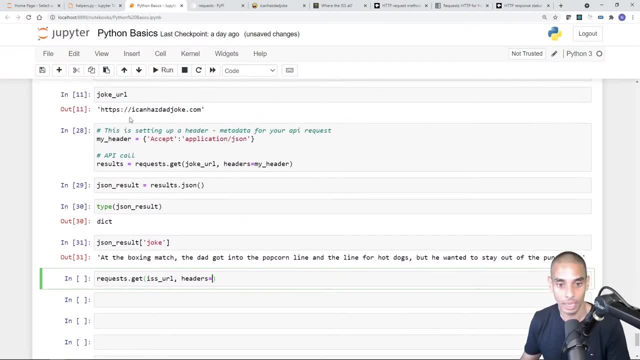 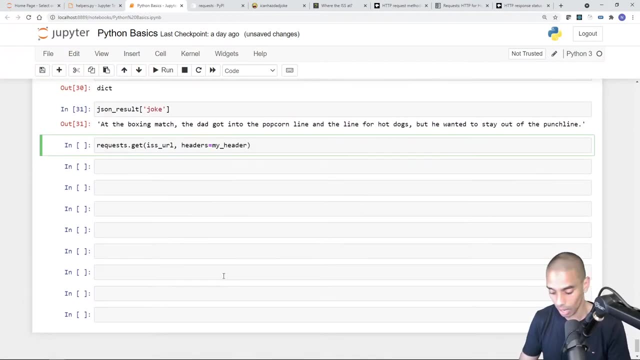 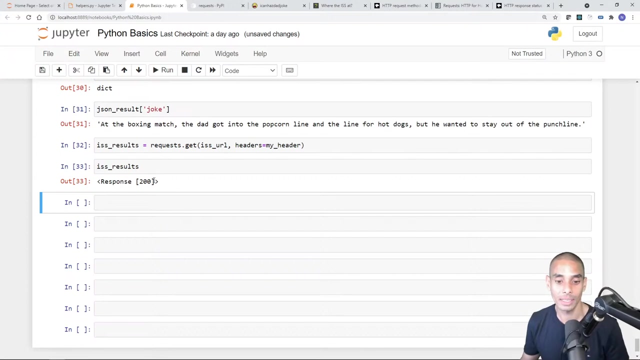 Headers equals. what are we setting it equal to? We're setting it equal to my header. So from over here, And we're going to store this inside of a variable called ISS underscore results, not in caps, Cool. So that looks like it's run No errors. yet If we type in ISS results, we've got a response status code of 200.. 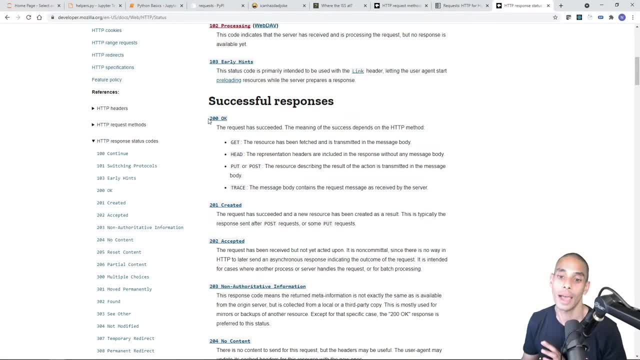 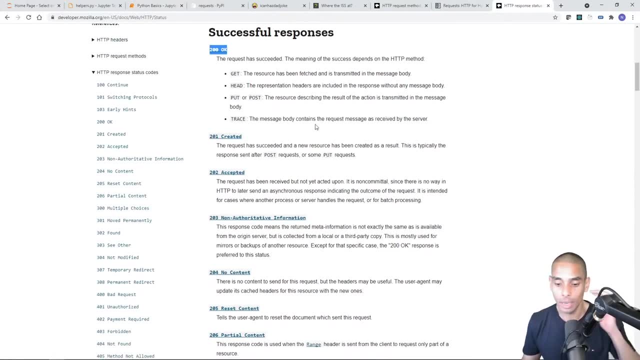 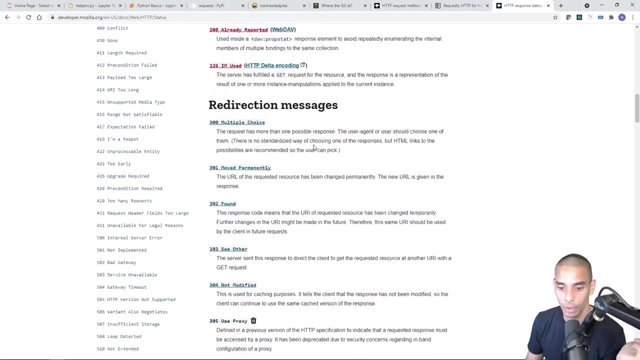 Remember a response status code of 200 is OK. Again, super lackluster and chill, It's just OK, But at least it's not some of the other ones that you might get. if it's not okay or not happy with you is 400.. 400 or 404.. I think it's 404.. 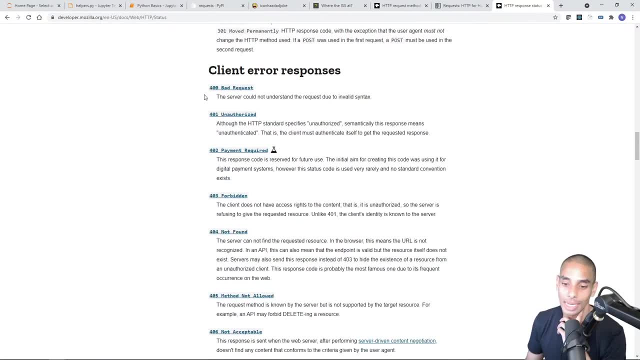 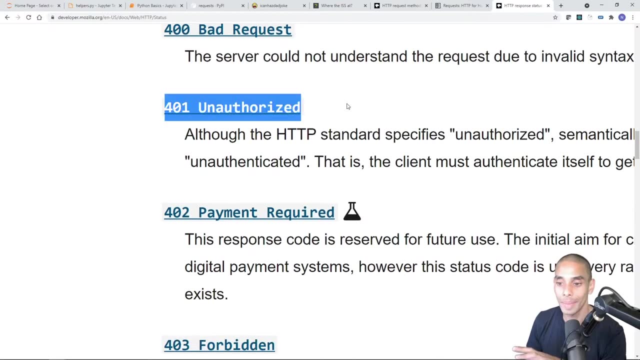 Alright, 400 is a bad request, So these ones are the ones that you need to look out for if you get this. So 400 is a bad request. Let me zoom in on this. 400 is bad API bad. 401 means you're unauthorized, so this typically means that you need to authenticate to the API. 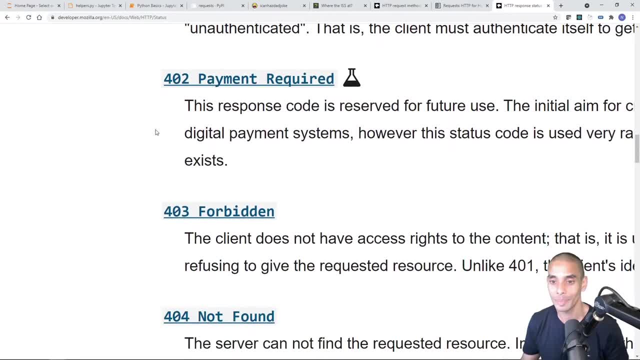 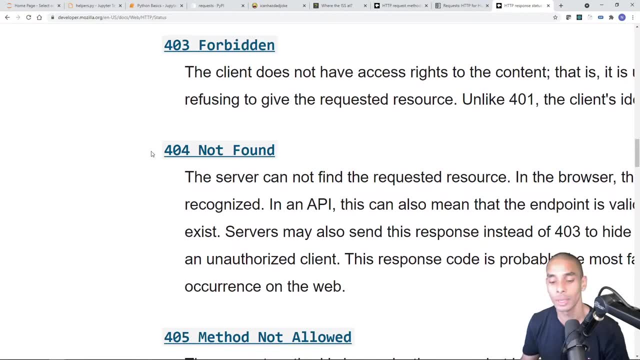 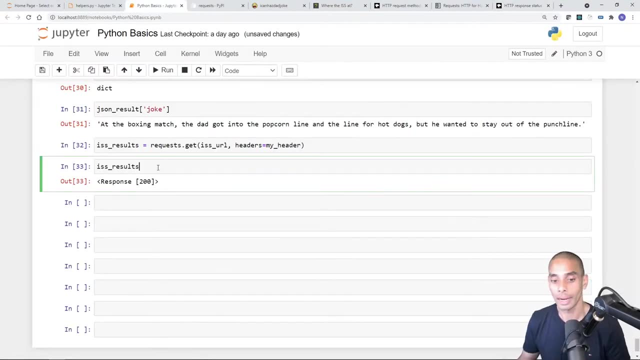 so pass your password or a token. 402 means payments required, 403 means it's forbidden, 404 probably means you've got the API endpoint wrong or it's not found, and so those are just some others that you might encounter on your journey with APIs. cool, what are we doing now? all right, 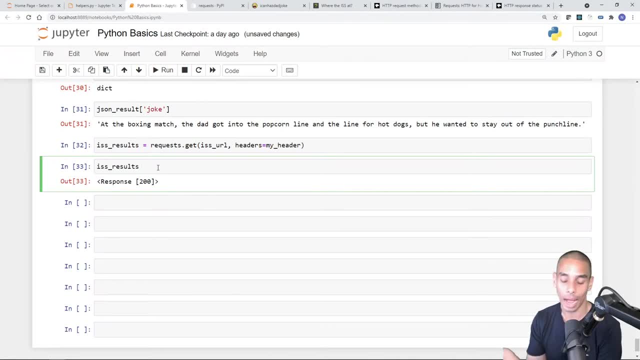 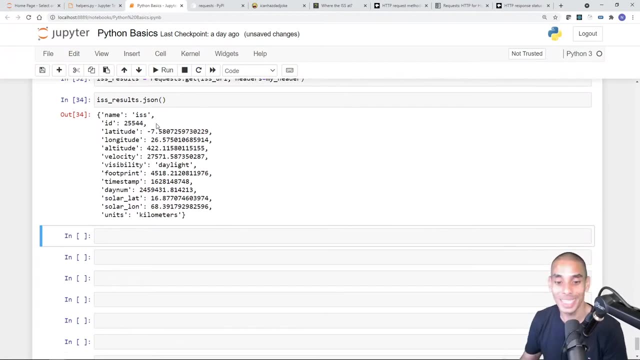 so we've gone and checked our ISS results. now what we want to do is we want to unpack our results, so we're going to type in dot JSON and that is our ISS stuff now return. but this is so cool, I'm absolutely in love with this. so you get a bunch of stuff back, so you get the name of the satellite. 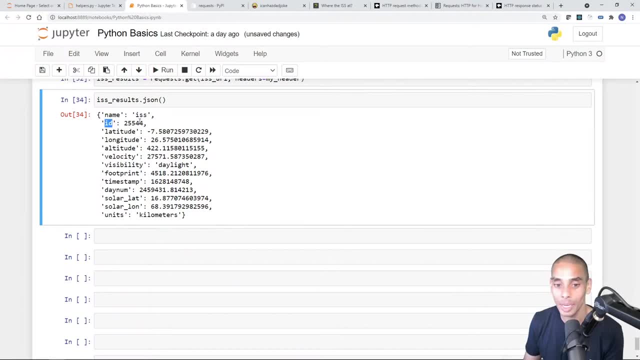 that it's actually tracking. in this case it's ISS. you get the satellite number, so 25544, yet it's latitude, it's longitude, it's altitude, it's velocity, it's visibility. so right now it's in daylight, it's footprint, it's time stamp, the day number, the solar latitude, solar longitude as well. 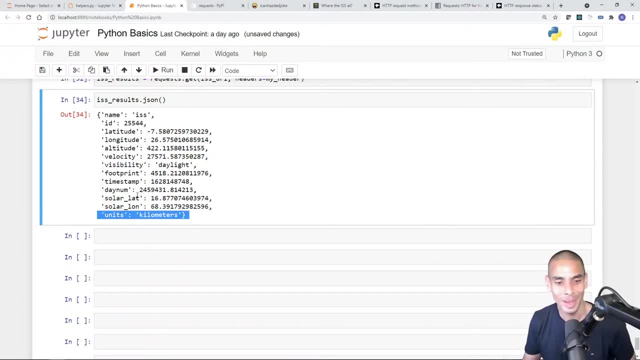 as the units that it's currently reporting in, so in this case it's kilometers. pretty cool, right? so there's a whole bunch of other APIs out there that you can start going out and exploring. there's a ton of stuff that you can do with this um and that really just summarizes what's possible with packages, so we haven't had to write any of the 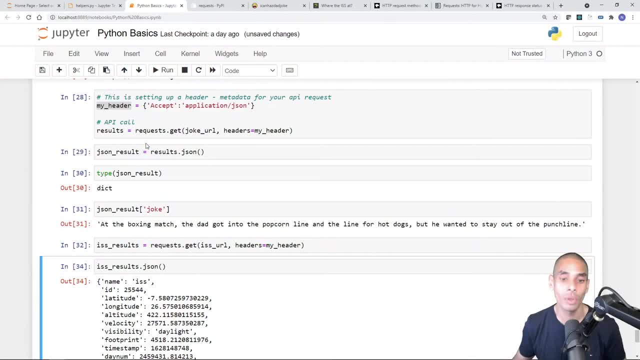 complex mechanics in the background to go and make an API call. the request package handles all of that complexity for us and really makes our life a whole heap easier. so let's recap what we've gone through and then we'll take some questions. so we've gone through. 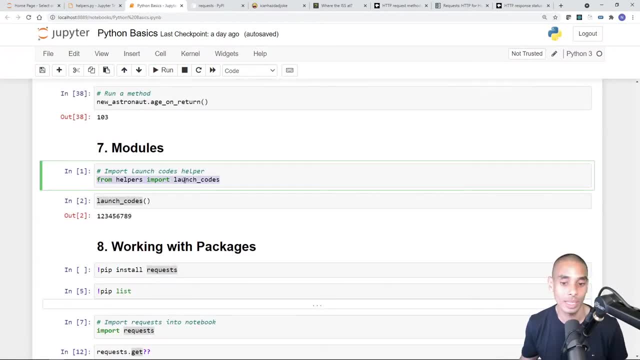 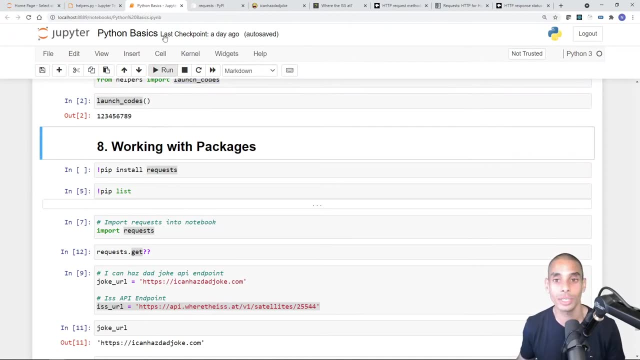 some modules and remember we can import some modules from another file, so in this case we're importing launch codes from our helperspi file up here. we then took a look at how we can work with packages and remember you can take a look at all the different packages that are available by 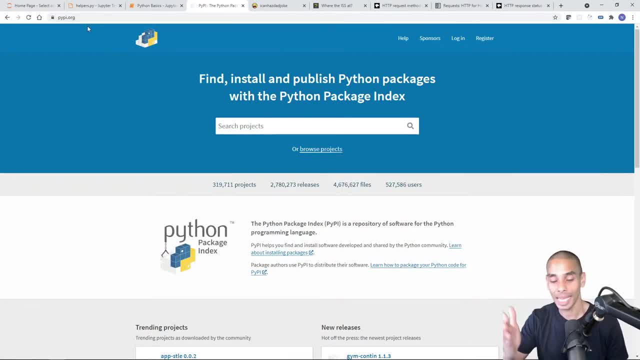 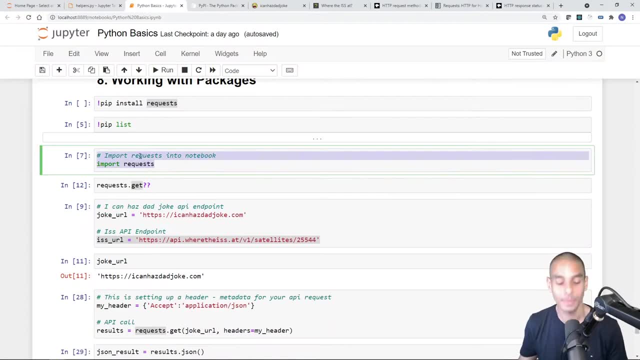 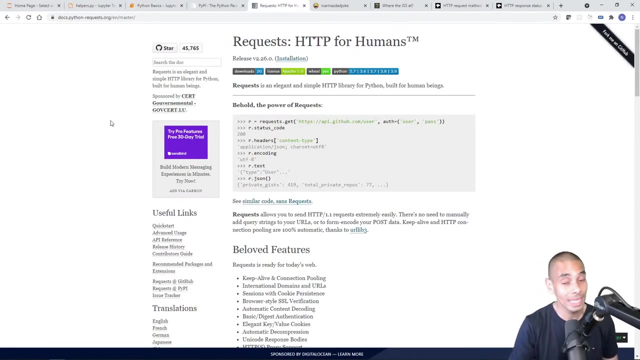 going to piorg. so that's pypiorg. and then we've also taken a look at one of the most popular packages, which is requests, and requests allows us to make API calls. so this is the request API documentation. really, really good practice to go and read the API documentation because it tells you. 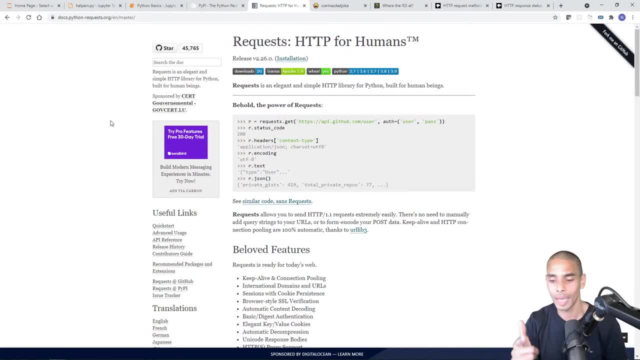 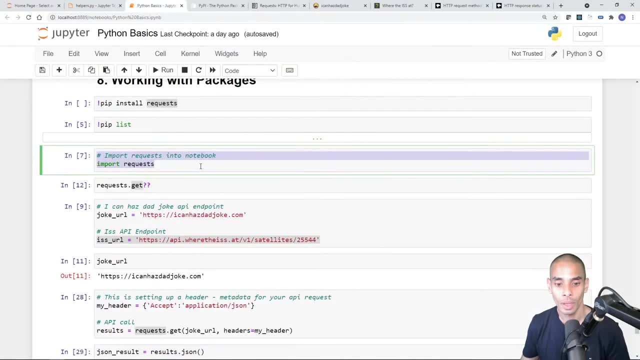 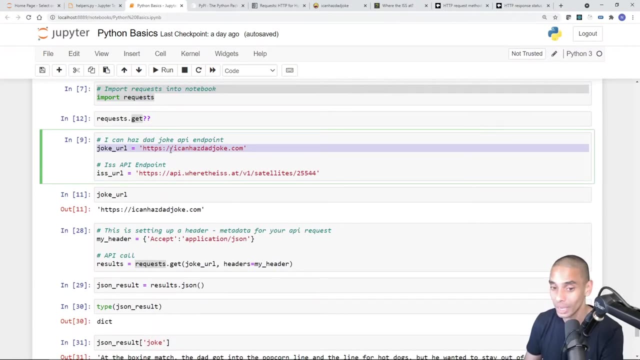 a lot about how the package actually works, not API documentation, package documentation. it's also good to read API documentation as well if you're using an API. uh, where are we now? then we went and set up two new URLs to go in, or two specific API endpoints to be able to go and make API calls, and then we 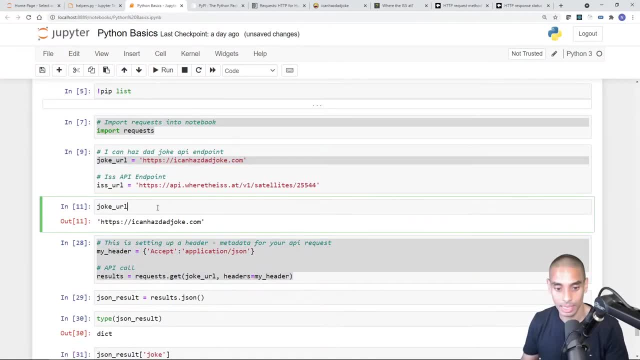 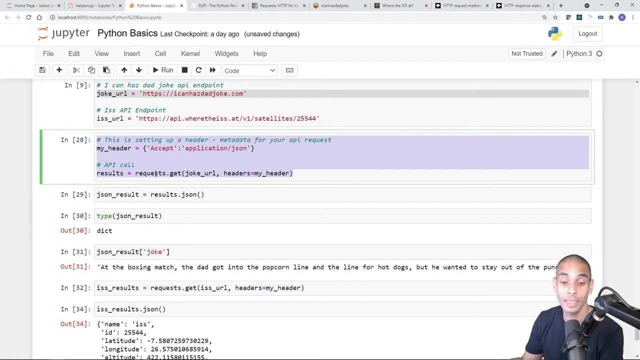 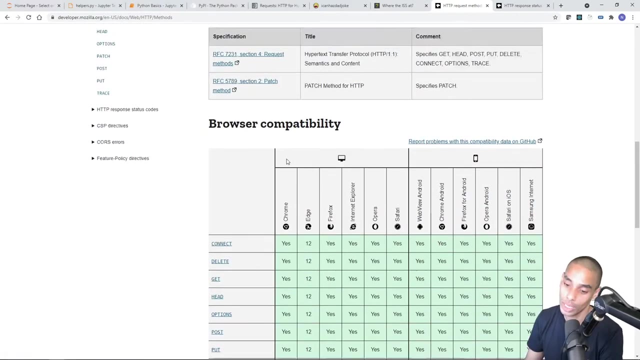 actually went and made our API calls there. let's actually clean this up, so I'm going to delete that. so these were API calls and, remember, one of the most popular methods, or HTTP request methods that you're going to use, is the get method. so this is a list of all the different types of HTTP request. 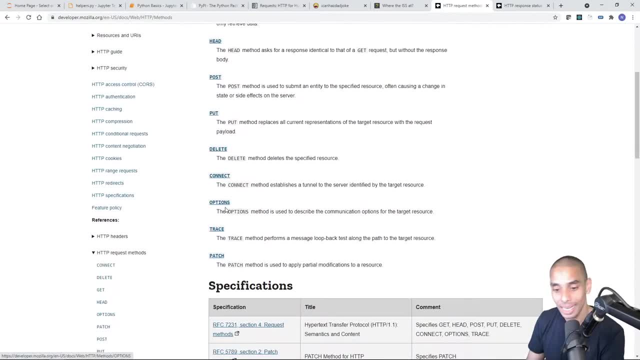 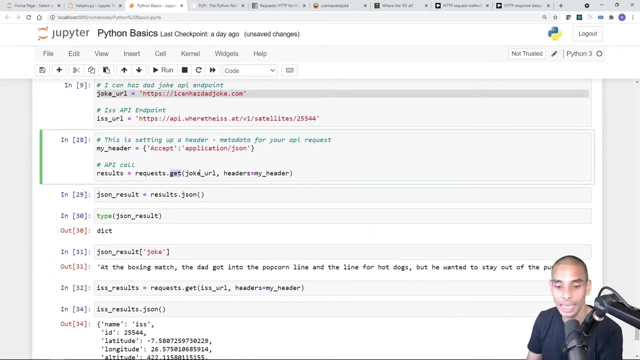 methods you might encounter. so get, head post put, delete, connect options, trace and patch. most often, you're probably going to be using get or put. in this particular case, we can pass through our URL as well as some keyword parameters, which in this case is headers. we can then go and. 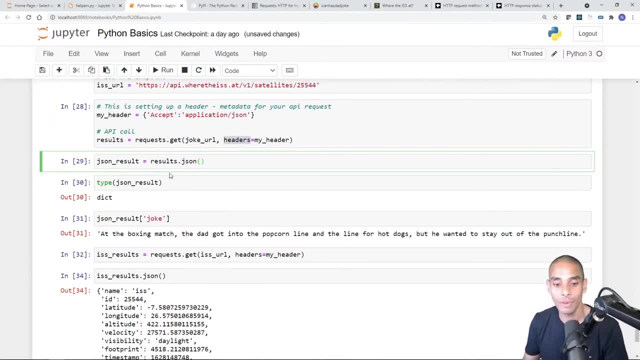 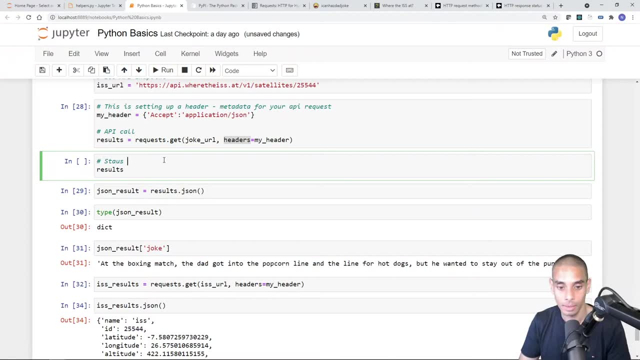 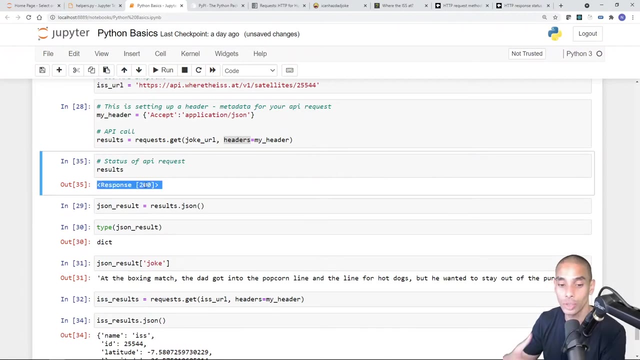 extract the results from our API call because, remember, by default, what we're going to get back is the status of our API call. so let's actually comment this. so status- status of API request. so remember, by default, when you actually just output the result, that's going to show the status. 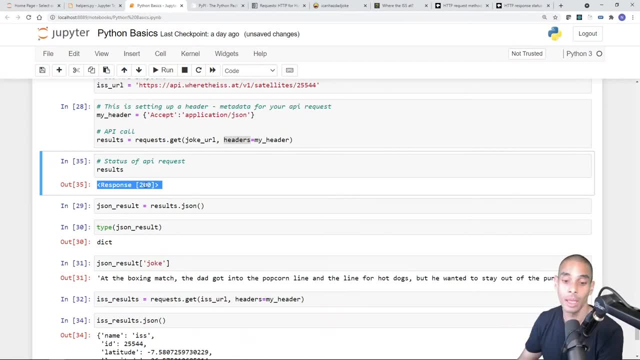 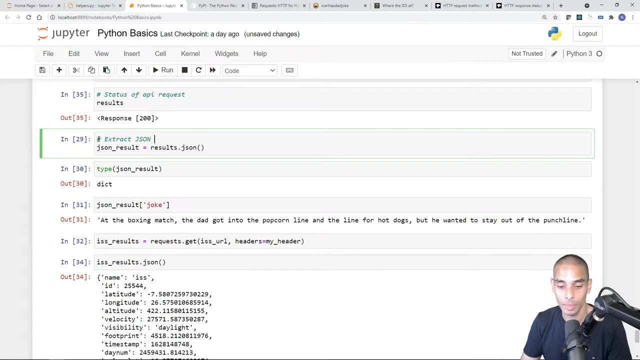 code. so in this case, a status code of 200 means it's okay. we can then go and extract the values from our API calls. remember, we're going to extract json results from the API. we can validate what type of data we're getting back in this case when we go and 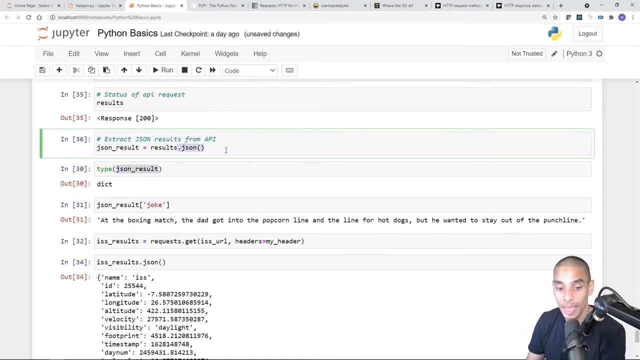 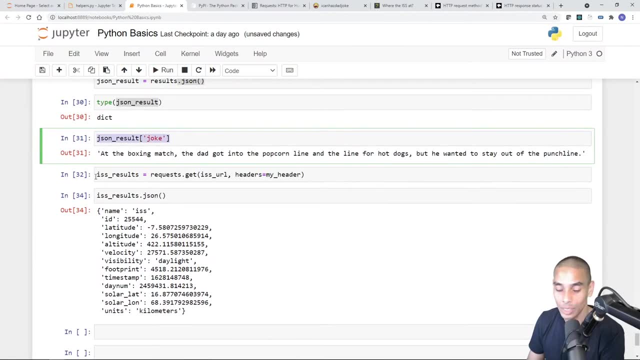 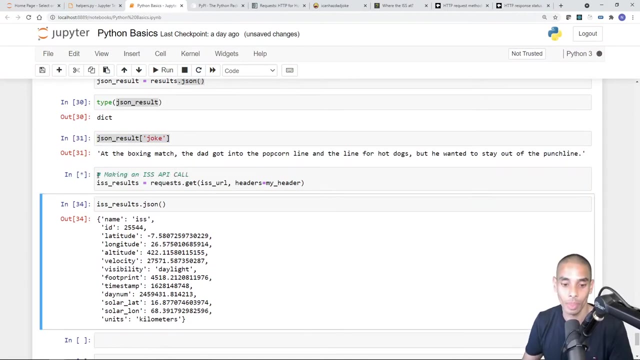 pass the json results. using thejson method, we're going to get a dictionary back. we can also unpack our dictionary to get our values back and in this case we've gone and made a iss API call. so, making an iss API call, remember there's a whole heap of different packages that are out there you can build. 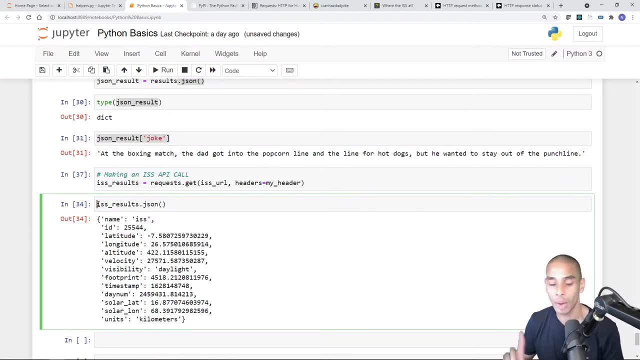 different modules. Some of my favorites, as I mentioned, are Pandas, PyTorch, TensorFlow. MediaPipe is another one that we've done a ton of work on. So if you want to go and check those out, what you'll see is in a lot of the videos that I build first up. we go about by handling. 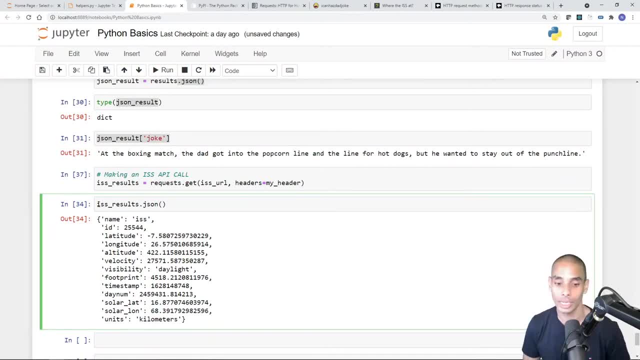 setting up different packages so that we can get started with our different projects. So this is super important when it comes to using these for data science. Alrighty, some time for questions. Oh wow, We've got a lot of questions here. 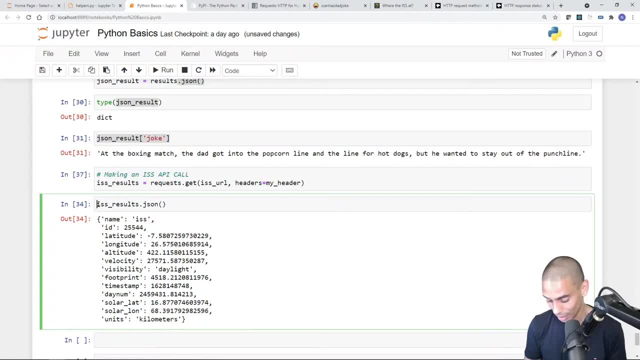 What's happening? Are you pleased to have you on the live stream, PowerCube? what up Manohar? what up Farun? awesome man, How you doing Ashish? What's happening? Dad jokes- Yeah, these dad jokes were absolute shocker, But I mean. 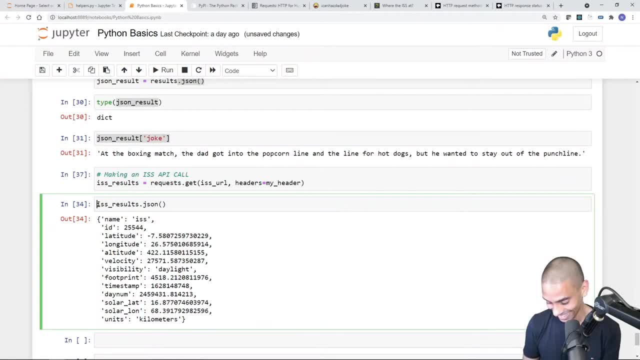 what can you expect? They're dad jokes. What else? Yeah, the ISS just flying around, PowerCube, who knows? Documentation is greater than Stack Overflow. I mean, Stack Overflow definitely has its uses. If you can truly understand and read all documentation, then that will make you an. 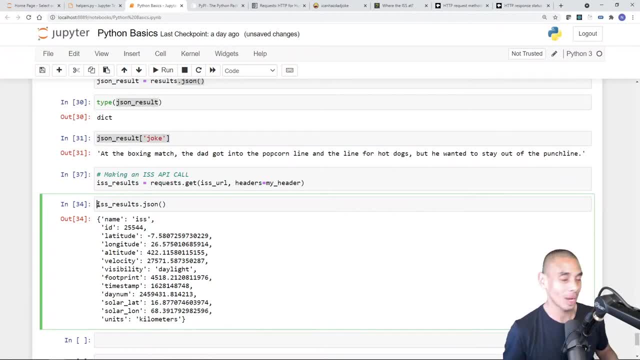 absolute, ridiculously amazing programmer. So half the time I barely read documentation like I'll just jump straight into it, But more often than not I find myself coming back to documentation, So it definitely comes in handy. This is a really good question, So. 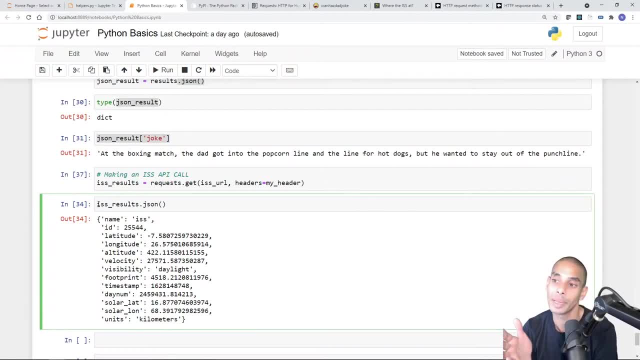 why would we use most APIs? Okay, so certain companies are going to actually render or share their data using an API. Now, a lot of the time, this is how they'll share their data with external organizations. Often, when you're dealing with data,